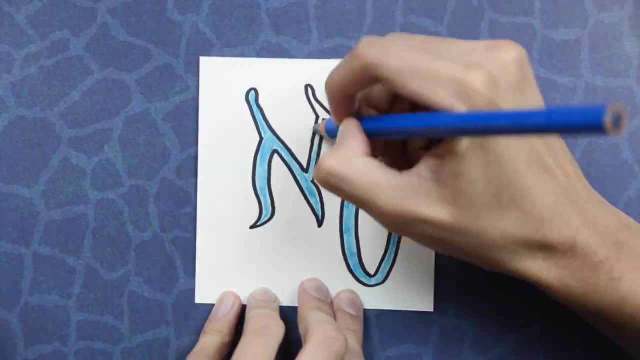 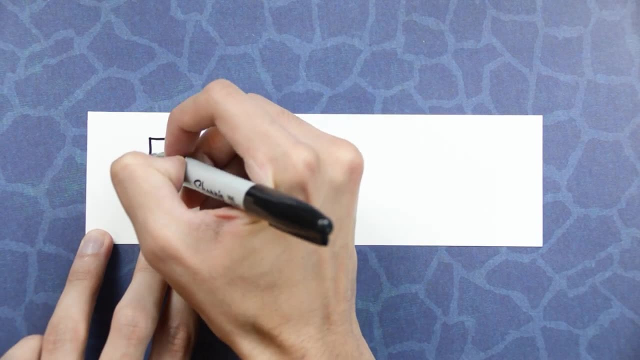 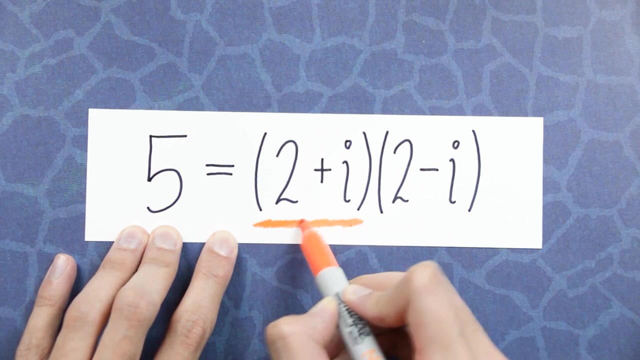 There's a very real sense in which 5 isn't a prime number, because you can write it as 2 plus i times 2 minus i. You can write it as a product of two numbers other than just 1 times 5.. This reveals something very interesting: Whether something is prime depends on the 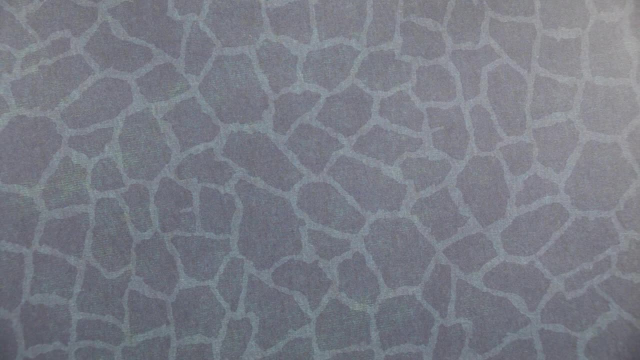 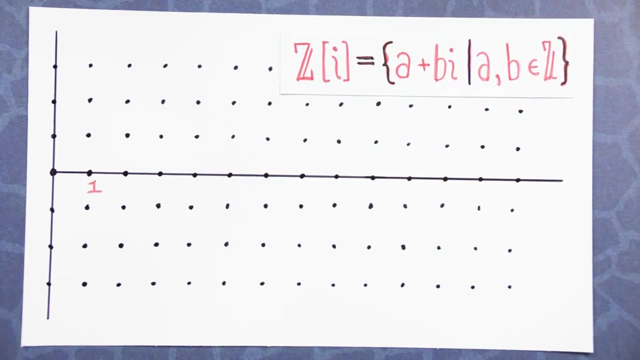 universe of numbers you're living in. What's happening visually is the following: Normally we work over the integers. that's the number line. Now we're working in a lattice in the complex plane consisting of all complex numbers with integer coordinates. You can write 5. 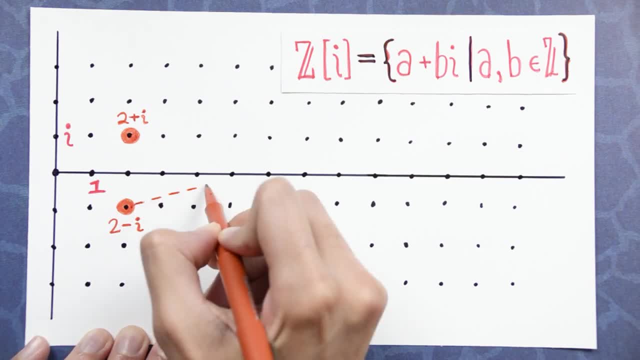 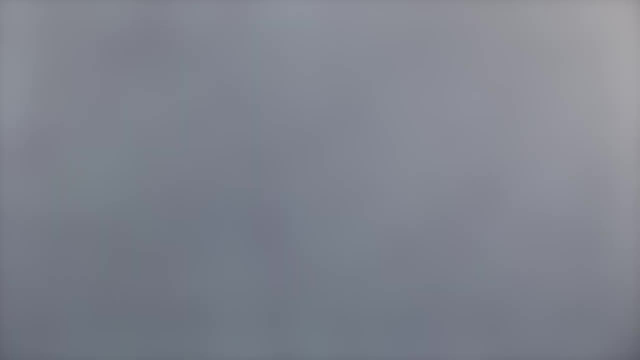 as 2 plus i over here, times 2 minus i over here. So in this number system 5 isn't prime. Our basic question in this video is as follows: How do the rules of number theory change when you extend your universe of numbers beyond the integers, The field of math that deals? 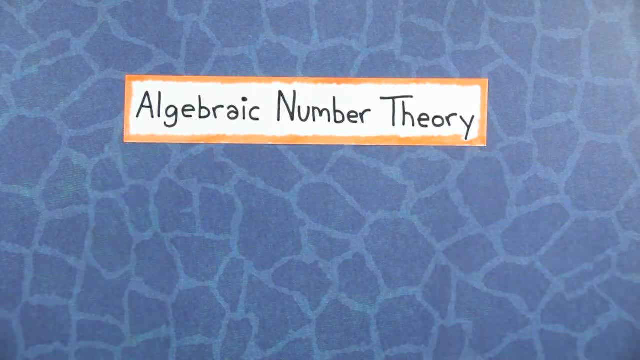 with this question is called algebraic number theory. In this video, we'll first introduce the basic concepts of this subject. This will allow us to enter one of the most beautiful branches of the theory of numbers, called Iwasawa theory. This is the branch of math. 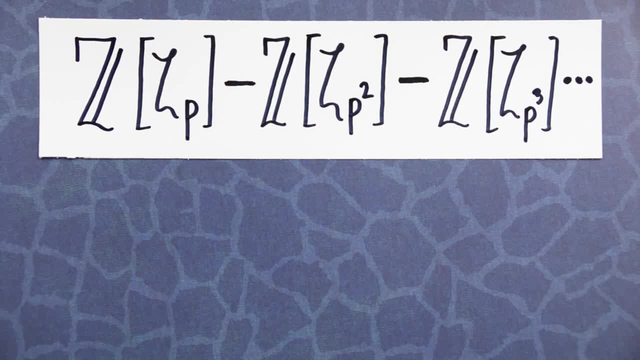 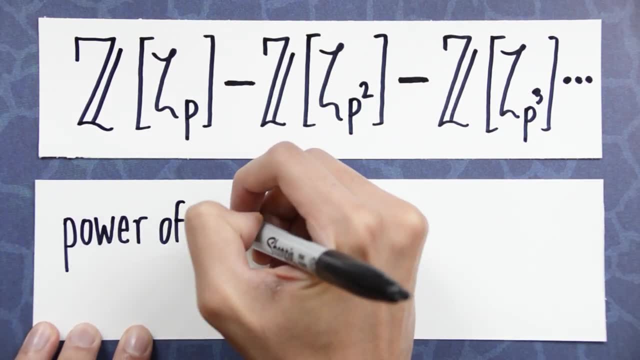 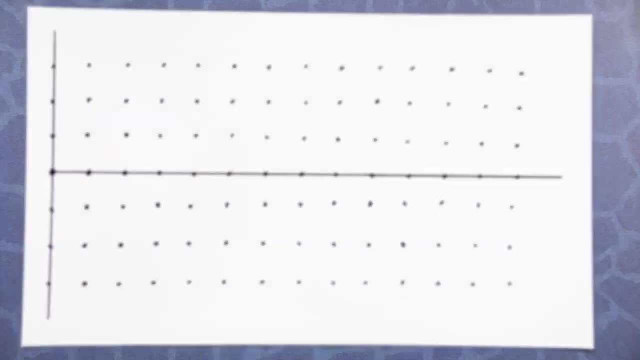 that does number theory in infinite hours. The culmination of this video is the foundational result of this subject, which very loosely describes how numbers factor into primes as you climb the layers of a certain infinite tower. It's honestly one of the most beautiful things in the world. Before we start, I'd like to introduce some helpful terminology. 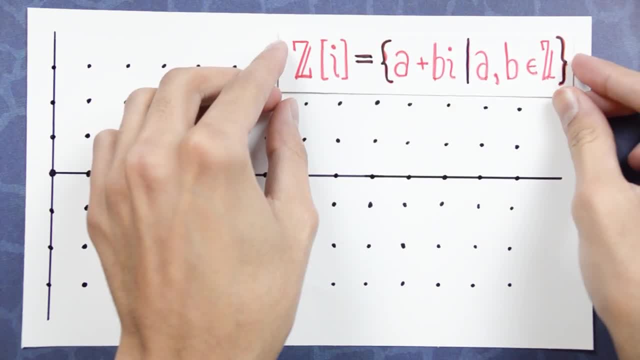 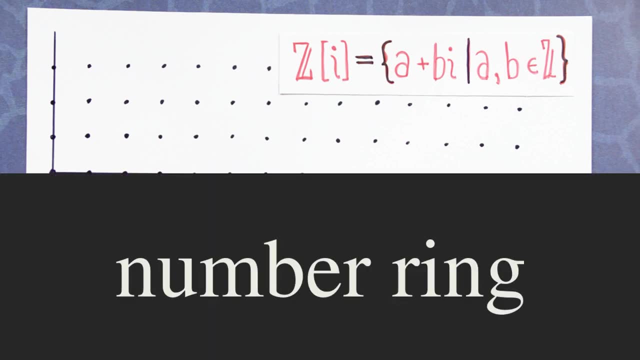 This number system that we saw is called z-adjoin i. It's the set of all complex numbers, a plus bi, such that a and b are integers. This is an example of something called a number ring. A number ring is a universe of numbers like the integers. Now I'm not going to give a. 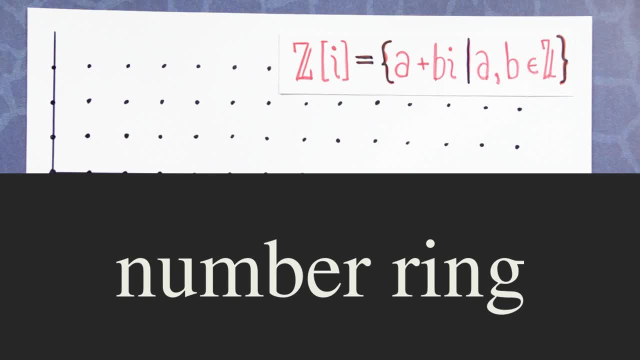 precise definition in this video. so the viewpoint we're taking is: you know it when you see it- The main theme when studying number systems like this is to know what the numbers are. The main theme when studying number systems like this is to know what the numbers are. The main theme when studying number systems like 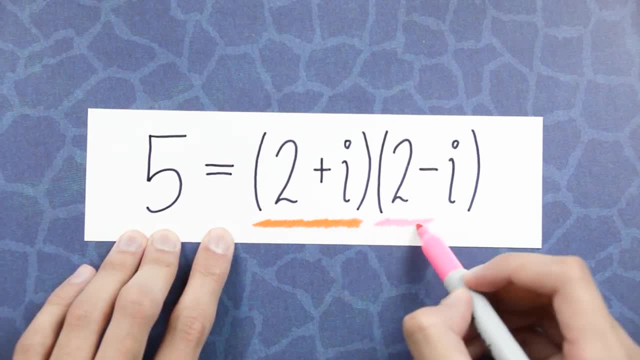 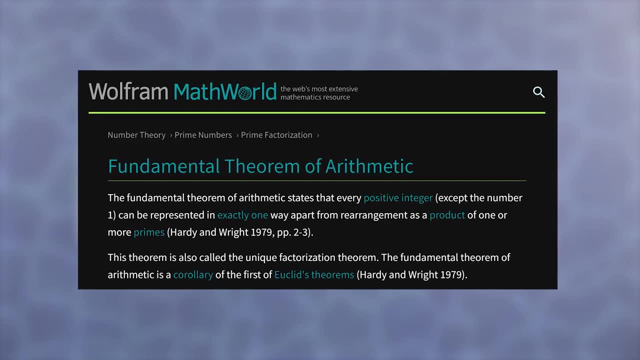 these is that many things that we take for granted over the integers aren't true over number rings. We saw one example: 5 is no longer a prime. Another one, which is more serious: Over the integers, it's a fact that every number can be factored uniquely as a. 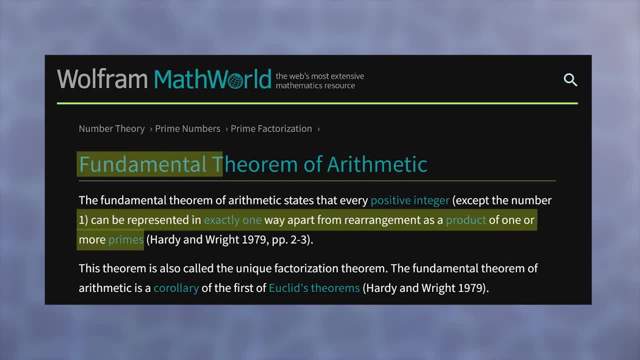 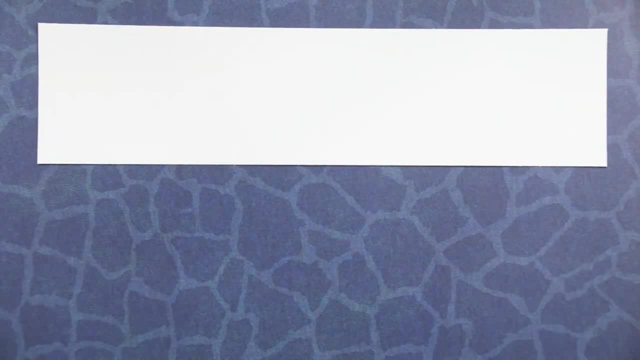 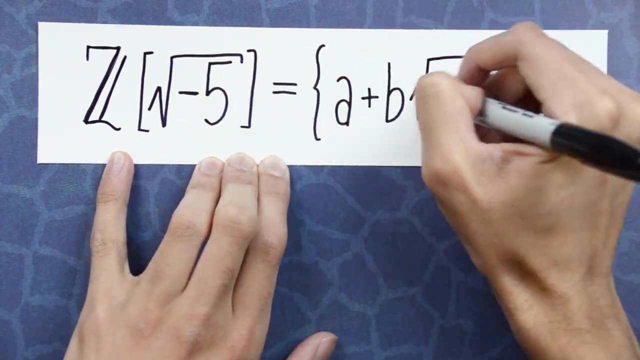 product of prime numbers. This is often called the fundamental theorem of arithmetic, because it's just so important. This fails quite spectacularly in other number systems. For example, consider the ring z-adjoin, the square root of minus 5.. The set of all complex numbers, a plus b, root minus 5, where a and b are integers. 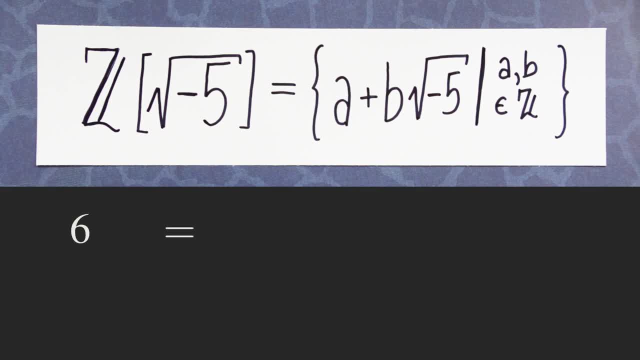 You can factor the number 6 in two ways. On one hand, you can write it as 2 times 3,, but you can also write it as 1 plus the square root of minus 5 times 1 minus the square root of minus 5.. So 6 factors as a product of primes in two different ways. Likewise, the number 21. 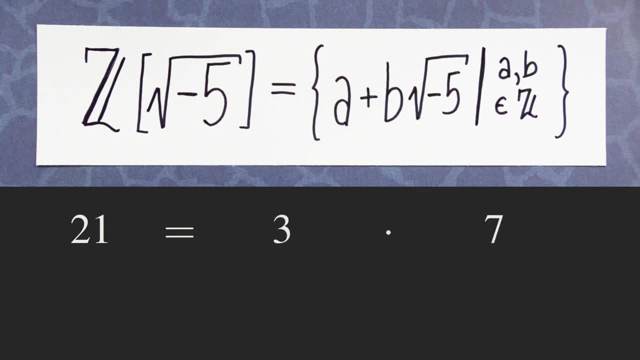 factors into primes in two different ways: 3 times 7, and four times root minus five times four minus root minus five. I want to stress: the problem here isn't that you can't factor numbers into primes. you totally can. rather, you can't do so. 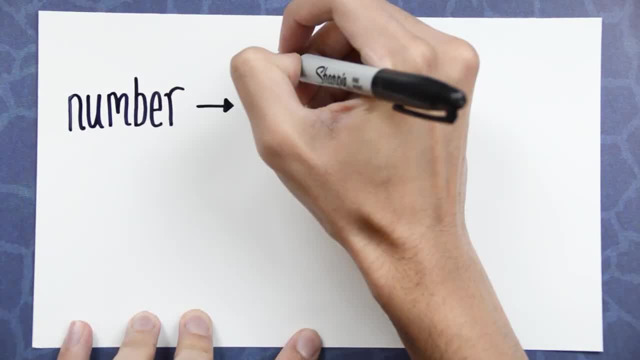 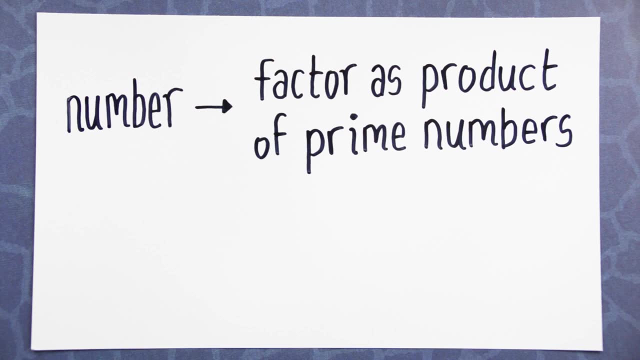 uniquely. This somehow suggests that looking at numbers and factoring them into prime numbers isn't the right way to look at things. The starting insight of algebraic number theory is, instead of looking at a single number, look at the set of all multiples of that number at the same. 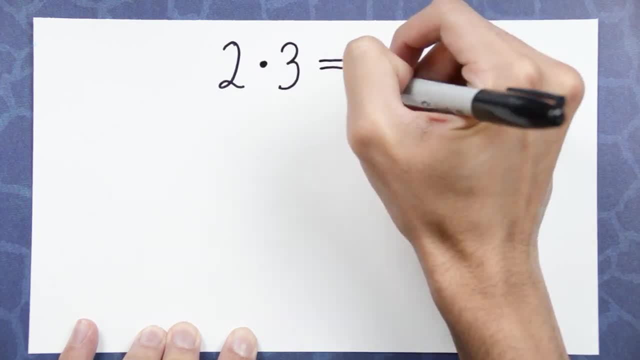 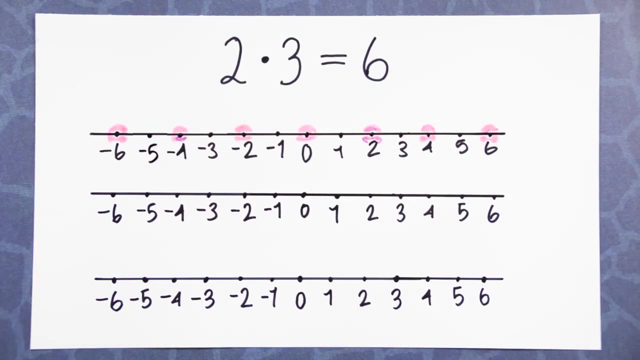 time. As an example, consider the equation: 2 times 3 equals 6.. So, instead of looking at the number 2, look at the set of all multiples of 2 at the same time, Instead of looking at the number 3,. 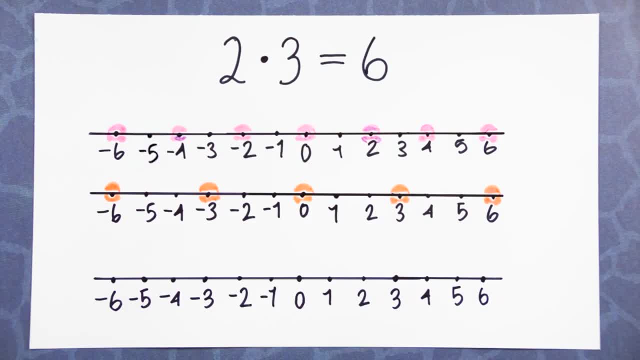 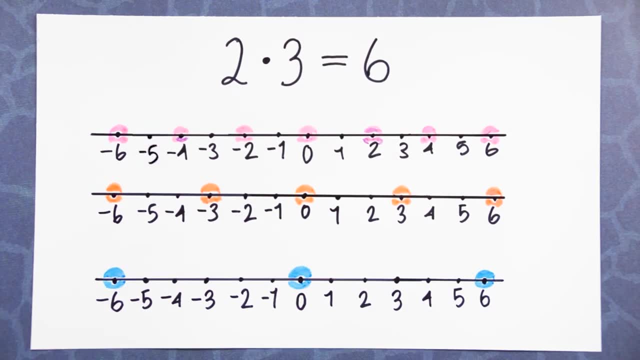 look at the set of all multiples of 3.. Now, if you multiply all the numbers here with all the numbers here in all possible combinations, you get this. Notice that the thing at the bottom is the set of all multiples of 6.. This allows us to interpret: 2 times 3 equals 6.. 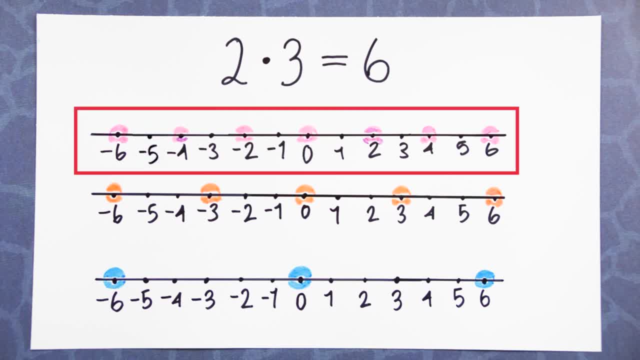 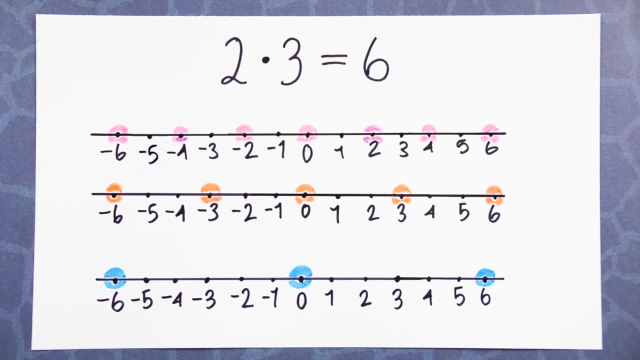 If you take all the numbers here and you multiply them by all the numbers here, you end up with all the multiples of 6.. Now over the integers. I agree that this is a totally bizarre way to look at things, but this perspective is crucial to how we're going to think about 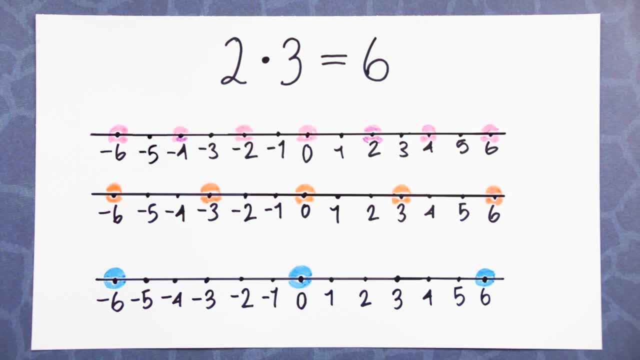 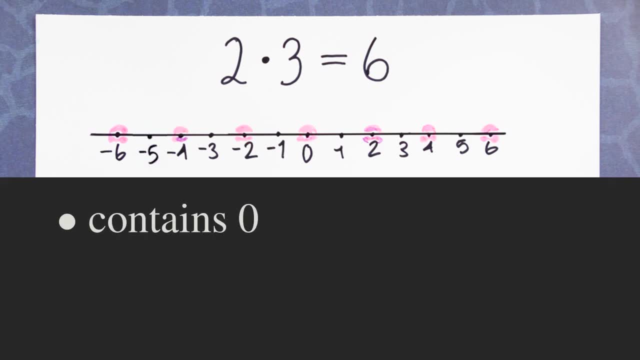 multiplication in higher number systems To see how it generalizes. we'll look at the properties of this set and make it into a definition. Notice that it satisfies these properties. First, it contains zero. Second, it contains zero. Third, it contains zero. Fourth, it contains zero. 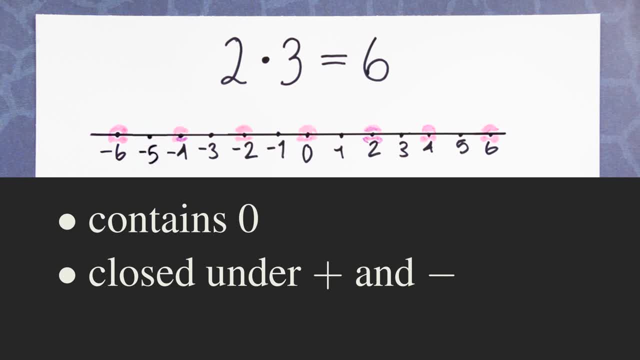 Second, it's closed under addition and multiplication. If you add or subtract any two multiples of 2, the result is a multiple of 2.. It is closed under taking multiples. If you have a multiple of 2, and you multiply it by any integer, the result is a multiple of 2.. 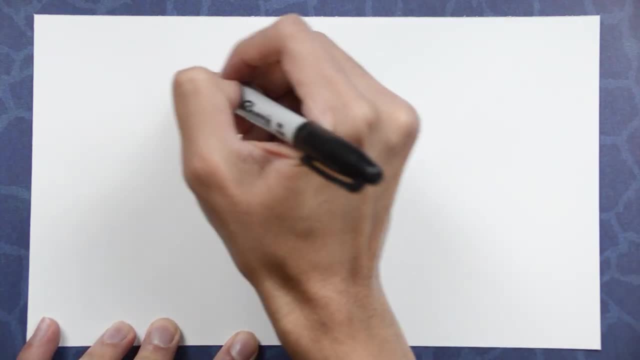 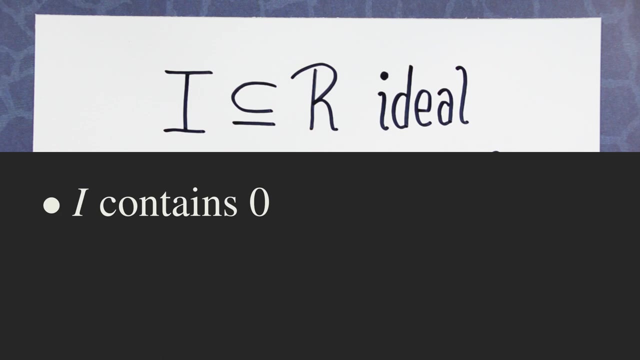 This motivates the following definition: If r is any number ring, an ideal is a subset i of r that satisfies these three same properties. First, i contains zero. Second, i is closed under addition and multiplication. And third, if x is an i. 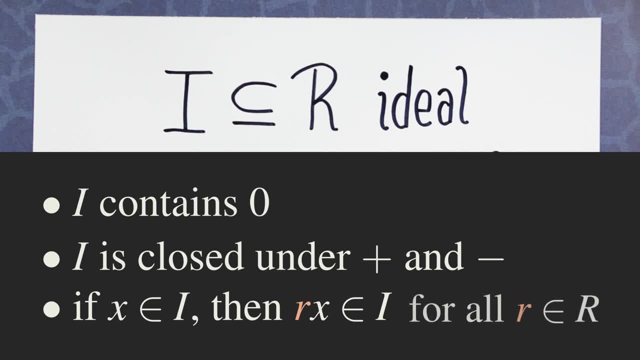 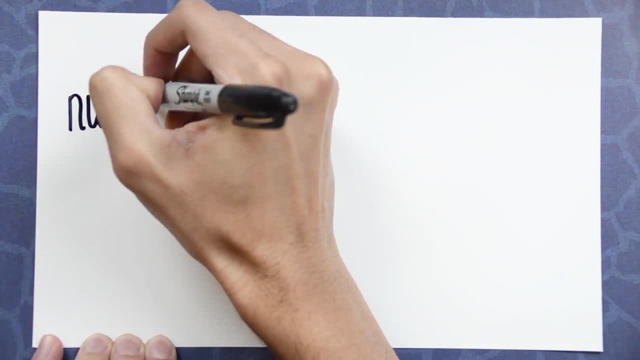 then r times x is an i for all. r in the ring, r Again. when I first saw this, it made my head want to explode, so let me just say where this is going. Originally given a number, we factored it into a product of prime numbers. 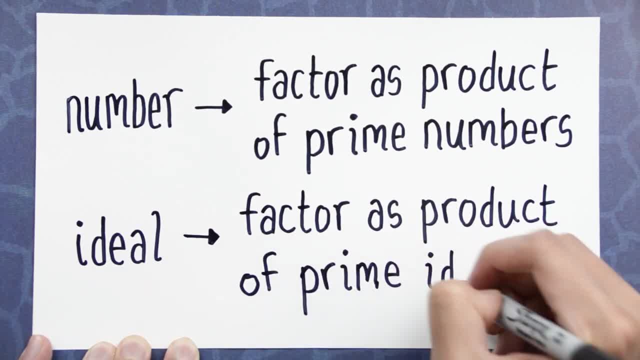 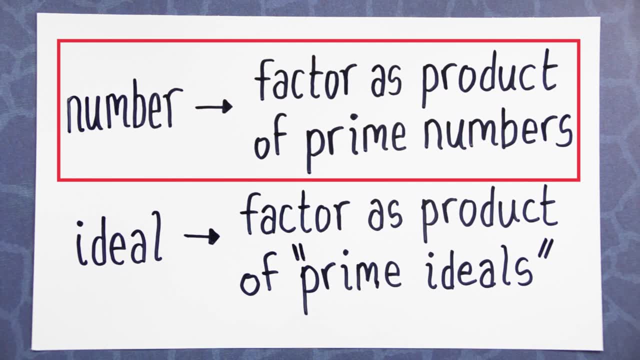 Now, given an ideal, we will factor it as a product of so-called prime ideals. For the first, we saw that unique factorization isn't true. It's not true that every number is uniquely a product of prime numbers. The point is for the bottom: unique factorization is true, Every ideal. 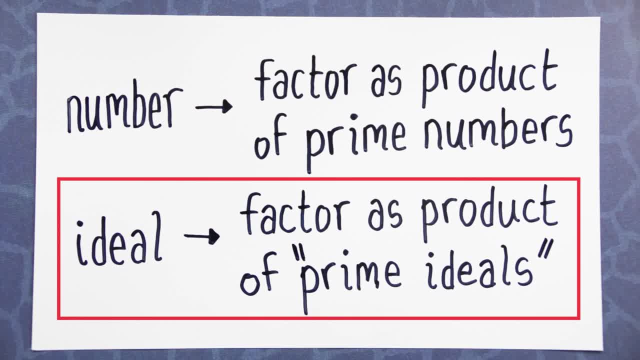 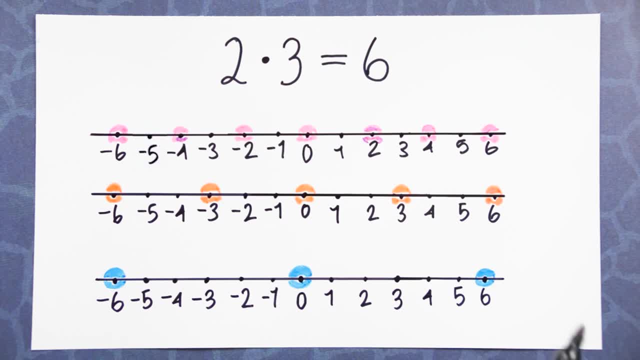 can be written uniquely as a product of prime ideals. That's the motivation for introducing ideals in the first place. First let's give some examples of what ideals are. In the integers, the set of all multiples of 2 is an ideal. It's written 2 with brackets around it. 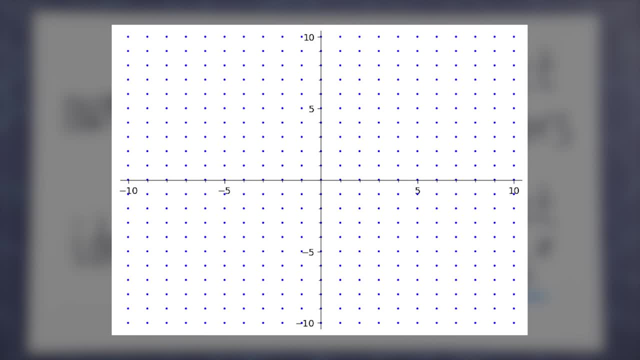 For another example, let's look at z adjoin. i Consider the point 1 plus i highlighted in red, Because an ideal is closed. under addition, any ideal containing this point has to contain twice that number and 0, and all integer multiples of that number As well. it should also contain: 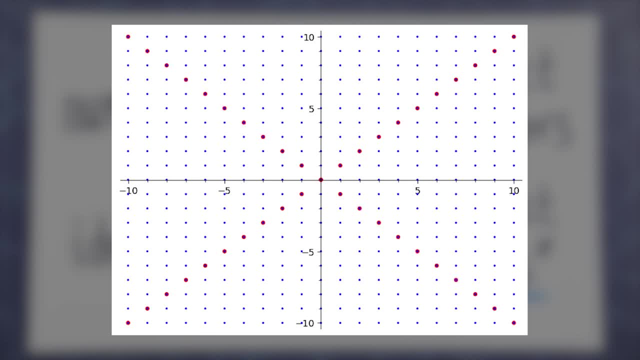 i times that number, which is this point over here, and then all integer multiples of that number. it should also contain all possible sums of these numbers, Filling in the gaps. you get this. This is the ideal written: 1 plus i. in brackets It's the set of all multiples of 1 plus i. 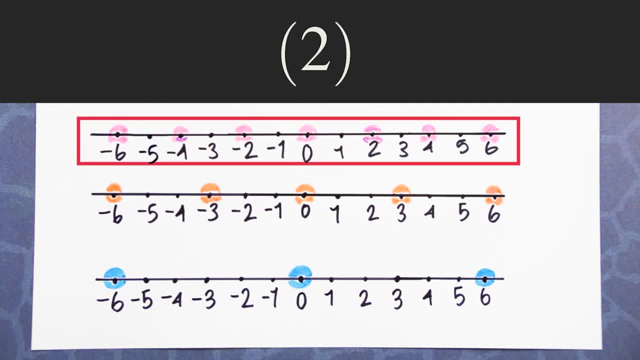 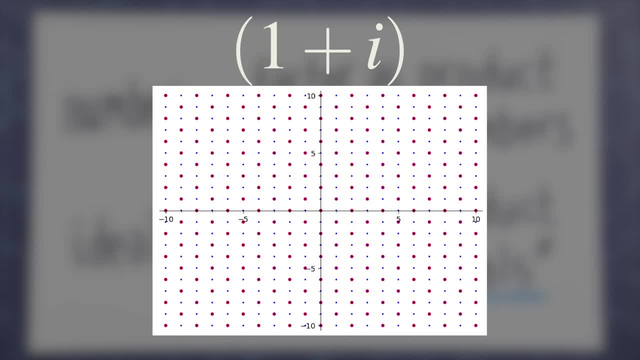 A word of warning. Both examples that we've seen the set of all multiples of 2, and the set of all multiples of 1, plus i have been the set of all multiples of a single number, But it's not true in general that all ideals have to be of that form, For example, 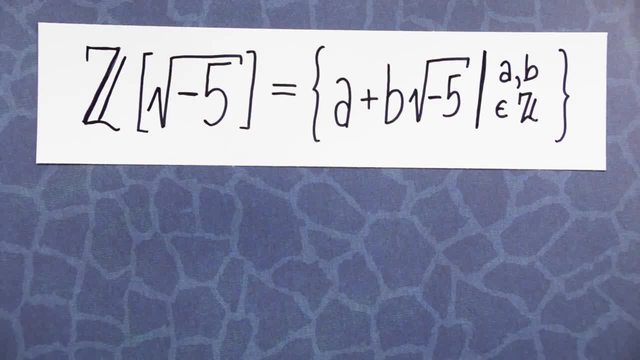 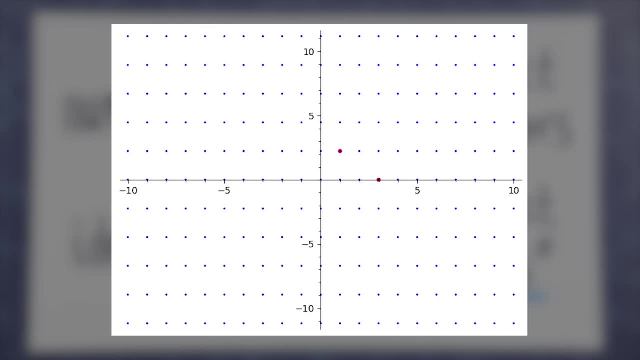 we looked at that ring z adjoin the square root of minus 5.. It looks like this: Now consider these 2 points. What's the smallest ideal containing them? Well, if it contains 3, it should contain all integer multiples of 3.. If it contains 1 plus root, minus 5, it should contain all integer multiples of that. 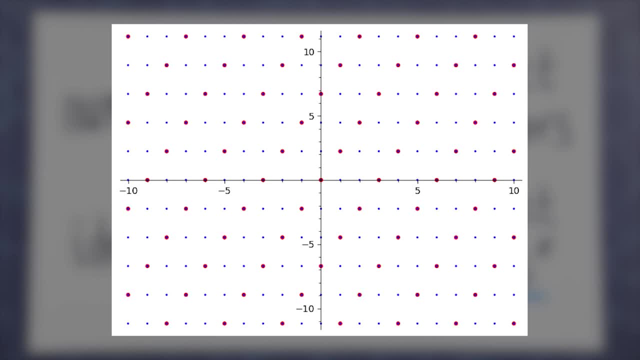 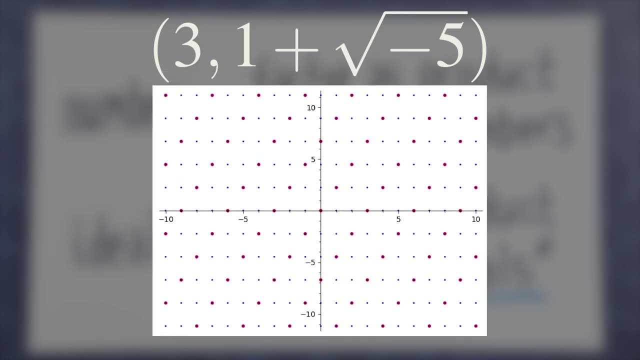 point. If you fill in the gaps, you get this. This is the ideal written: 3 comma, 1 plus root minus 5.. The ideal generated by 3 and 1 plus root minus 5.. Let's see how factoring into ideals as opposed to. 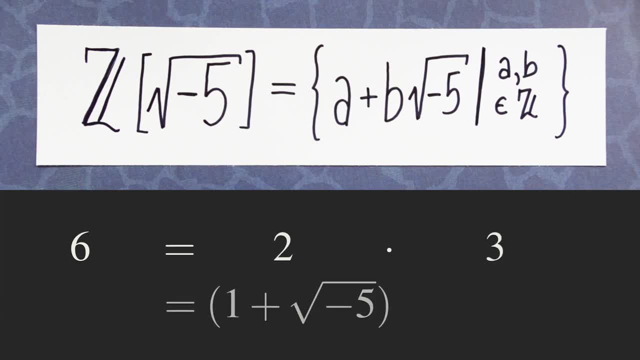 numbers fixes our older example. Let's see how factoring into ideals, as opposed to numbers, fixes our older example. So we saw that you can factor 6 in two ways. But now, instead of factoring the number 6, let's factor the ideal 6.. It factors as a product of 4 different prime ideals as follows: 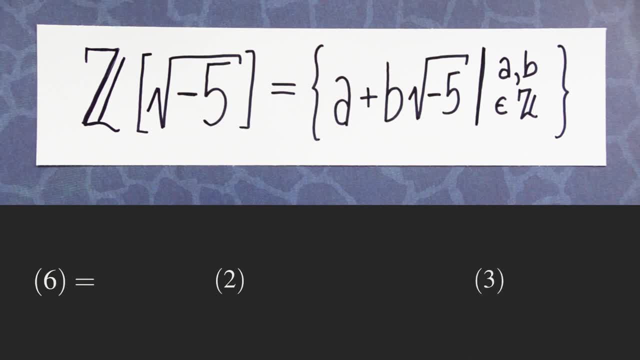 If you multiply the first 2, and then the second 2,, you get 6 equals 2 times 3,, our first factorization, And if you multiply them in a different order, you get our second factorization. So this whole time. 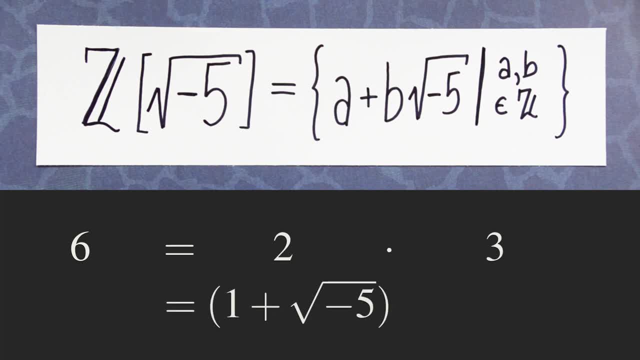 these two factorizations weren't actually different. There was just a deeper, underlying factorization into ideals and we were just grouping the terms in different ways. This is confusing, so it's worth summarizing what we've seen so far. We've seen that certain number 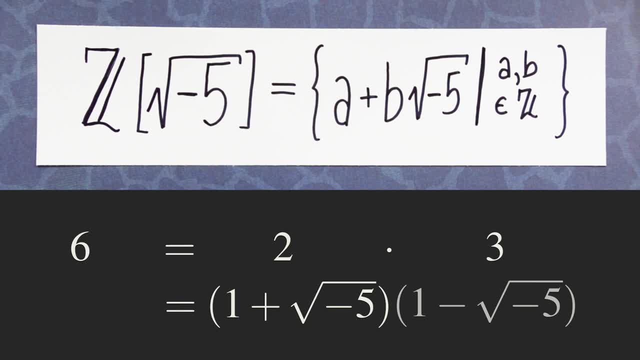 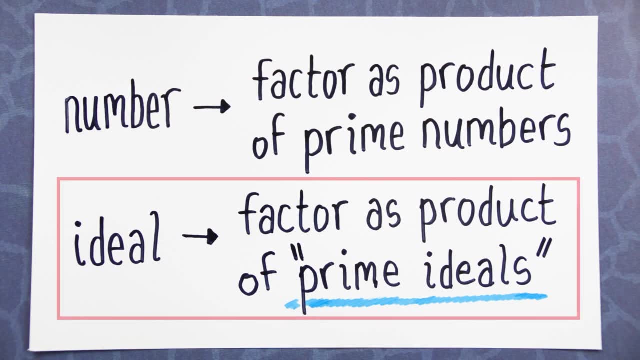 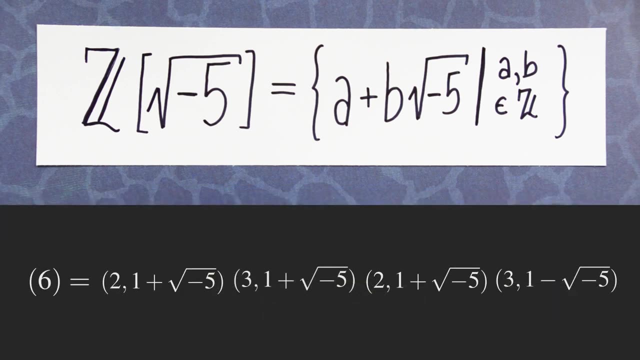 rings fail to have unique factorization into prime numbers, The fix was, instead of factoring numbers into prime numbers, factor ideals into prime ideals, And the way this fixes things is, whenever unique factorization into numbers happens to fail, there is always a deeper factorization into. 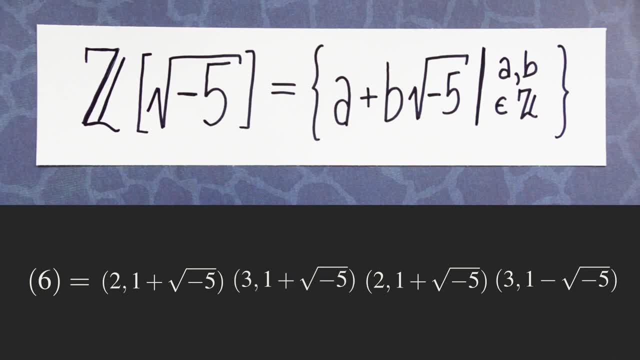 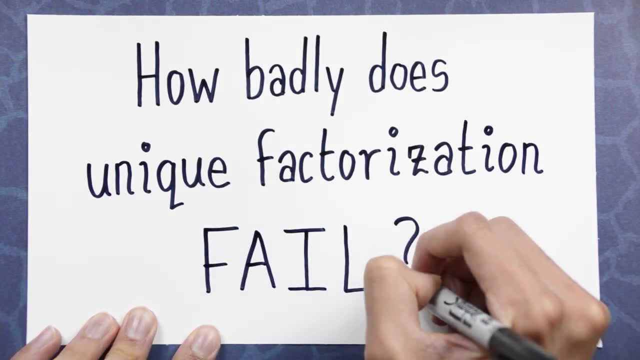 ideals that works. Now here's an interesting question: Given a number ring, how badly does unique factorization into prime numbers fail? This question will lead us to the punchline of this video. To answer this question, I'd like to introduce some helpful terminology. 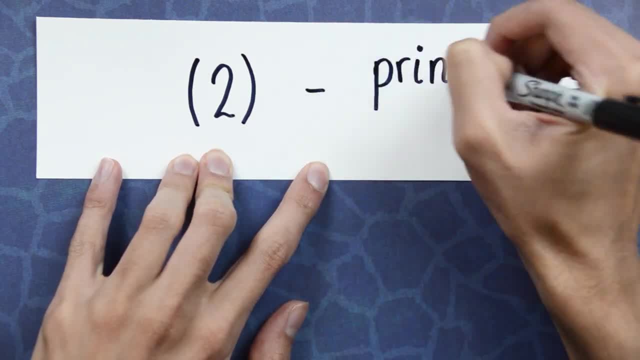 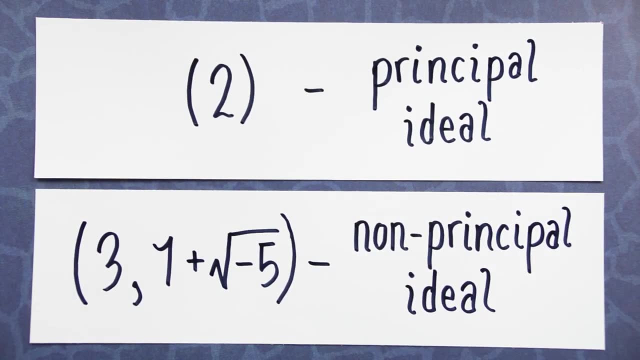 An ideal like this that's generated by one number is called a principal ideal. An ideal like this that's generated by more than one number is called a non-principal ideal. The point is: principal ideals are basically like numbers, You just write them with brackets. 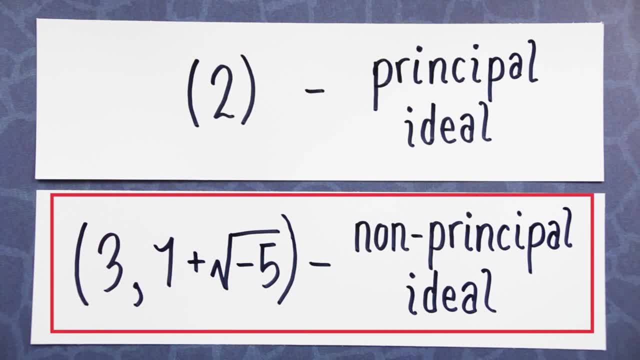 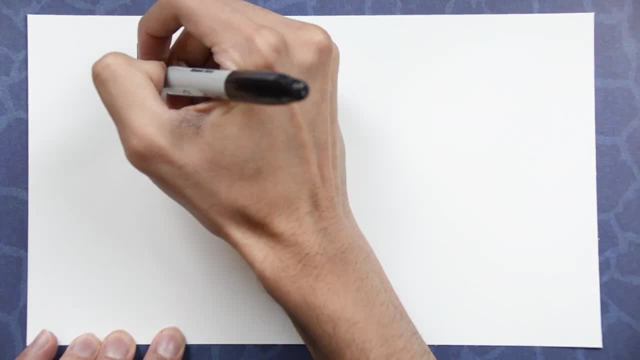 around them. But non-principal ideals aren't like numbers. They're things that you add in in order to restore unique factorization. So before we ask the question, given a number ring R, how badly does unique factorization fail? Now we can ask a more precise question. 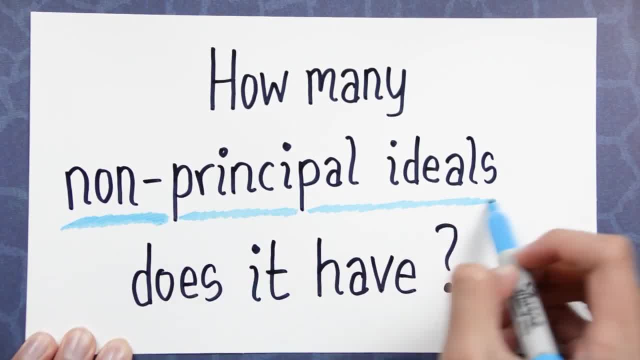 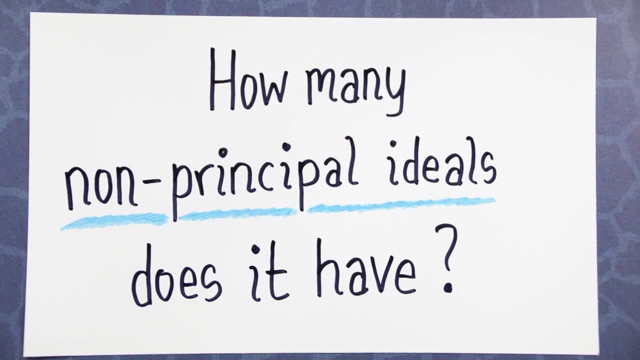 Given a number ring, how many non-principal ideals does it have? In other words, how many new ideals did you have to add in in order to restore unique factorization? Now, as it stands, this is not a well-defined question, because a number ring could have infinitely many non-principal ideals. 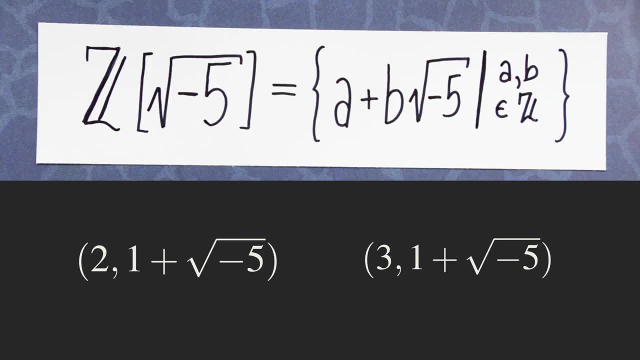 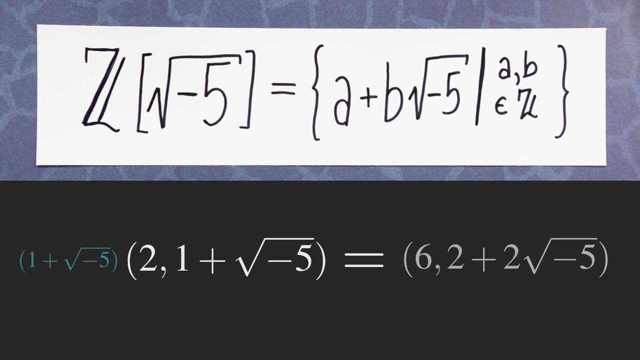 But there is a better way to quantify this. Consider these two prime ideals. It turns out that these ideals are scalar multiples of each other. In this case, that scalar happens to be 1 plus root, minus 5 over 2.. Likewise, it turns out that this ideal on the right is also some constant alpha times. the first: 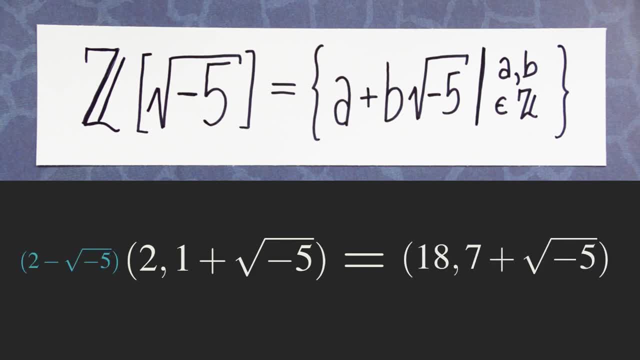 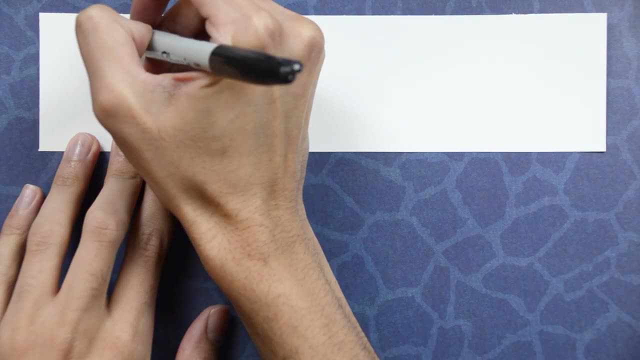 ideal. In fact, every non-principal ideal in this ring is a scalar multiple of this one. This ring has infinitely many non-principal ideals, but they are all of the same kind, so to speak. They all address the same illness in the underlying ring. But that's not always true. Consider the ring. 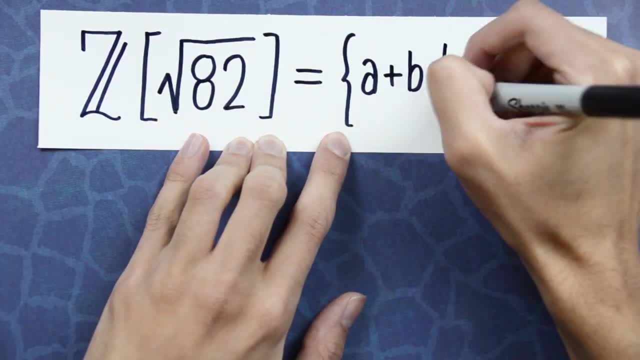 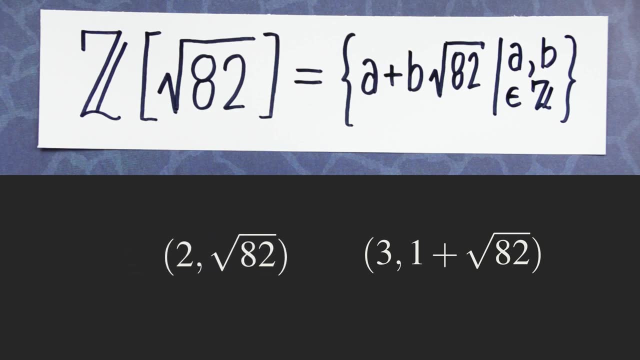 z adjoin root 82, which consists of all numbers a plus b. root 82, where a and b are integers Here. if you take these two ideals, then it turns out that they are not scalar multiples of each other. There is no constant alpha that makes this equation hold true. 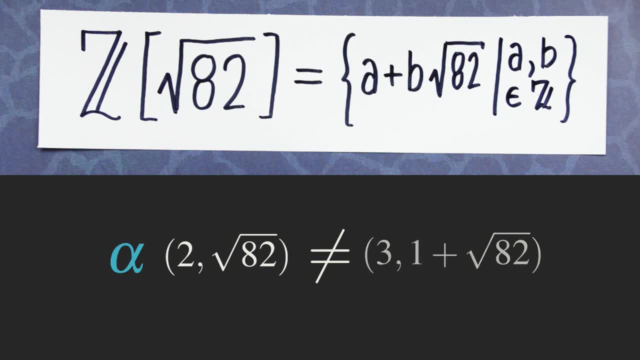 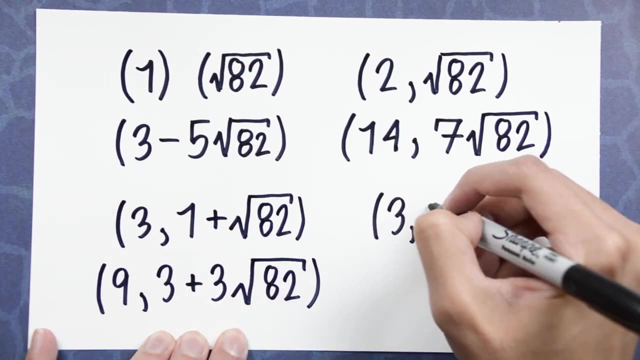 They are genuinely different kinds of ideals. Likewise with these two ideals, they aren't scalar multiples of each other either. So for this ring, you have to add in more than one kind of ideal in order to rescue unique factorization. To mentally organize this, let's do the following: 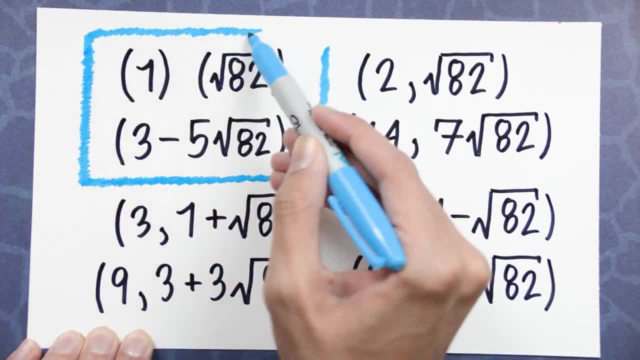 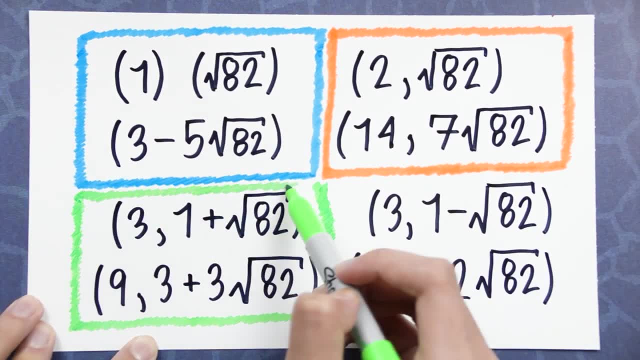 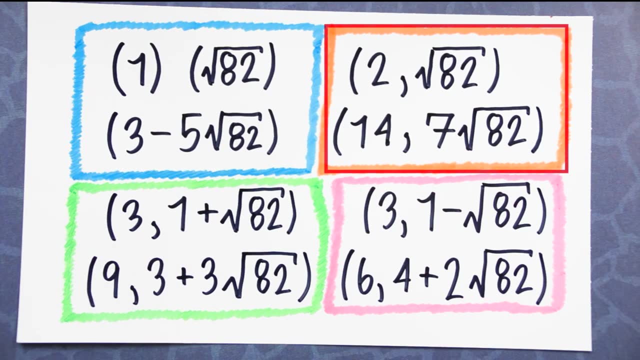 Put all the principal ideals of this ring in a box, Then sort the remaining ideals based on whether they are scalar multiples of each other. So this picture means all of the ideals living in the same box are scalar multiples of each other. This ring has four different kinds of 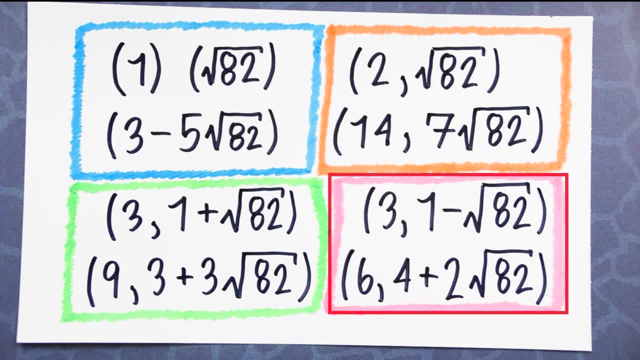 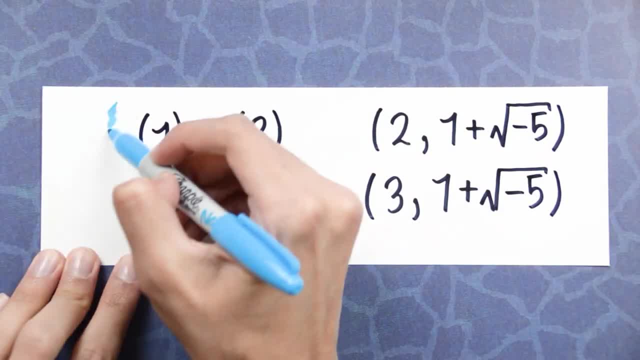 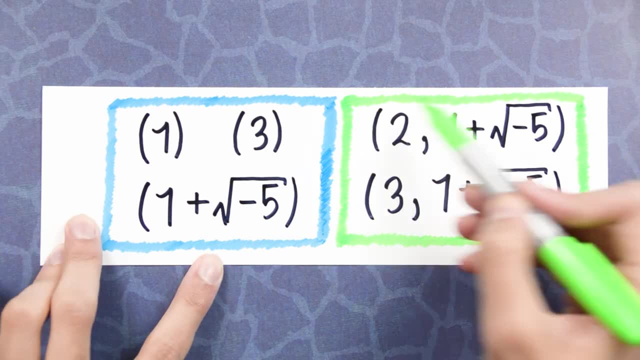 ideals. To fix unique factorization you had to apply four different band-aids. Compare that with the ring z adjoin root minus five. Here the picture is different. There are only two boxes: One for all the principal ideals and one for all the others, ie all the non-principal ideals are 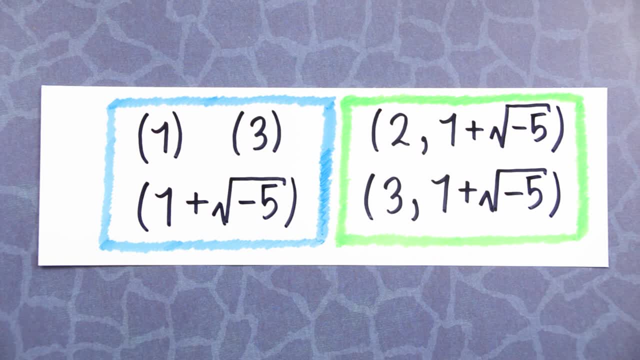 scalar multiples of each other. This ring has only two kinds of ideals. To fix unique factorization you only have to apply two band-aids. Some terminology- The number of kinds of ideals in a number ring, is called the class number of that ring. This ring has class number two. 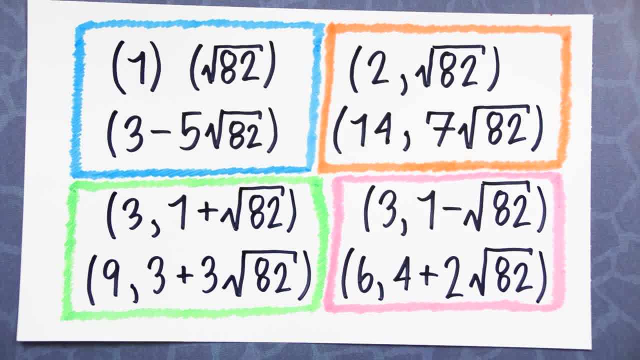 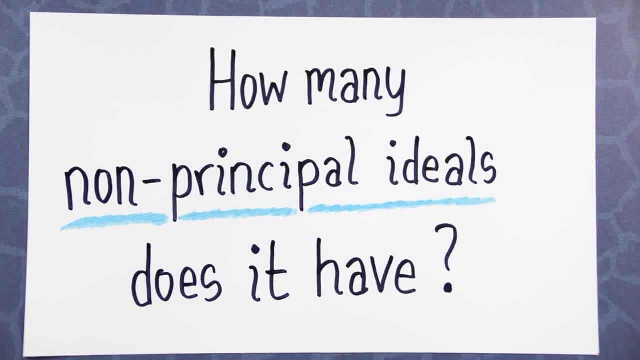 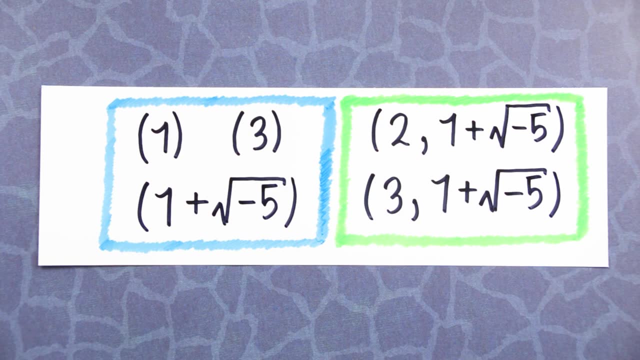 This ring has class number four. The class number answers our question: how many non-principal ideals did you have to add to recover unique factorization? It's a kind of proxy for how screwed up the underlying number system is. This ring has class number two. so it's kind of screwed up, but not too much. This ring has class. 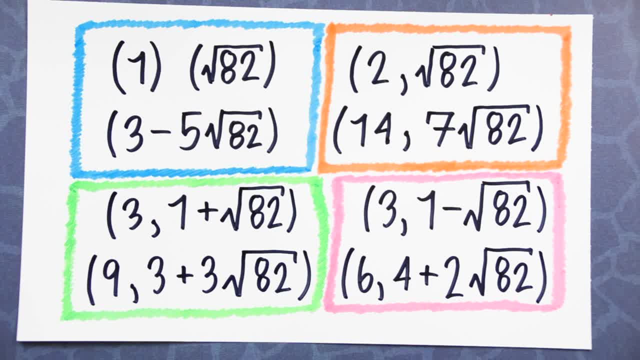 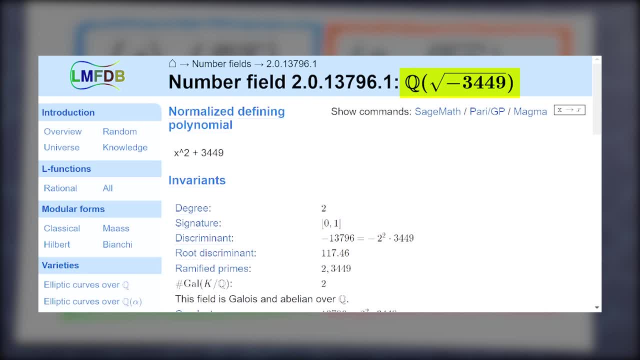 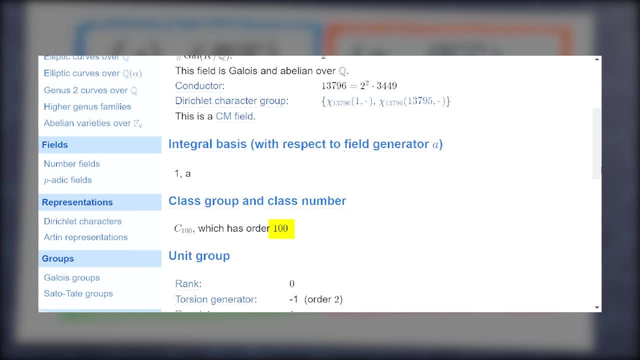 number four, so it's much more screwed up than the first one. In general, class numbers can get very large. For example, if you look at z adjoin the square root of minus three, four, four, nine, the class number is 100. There are 100 different kinds of ideals in this number system. 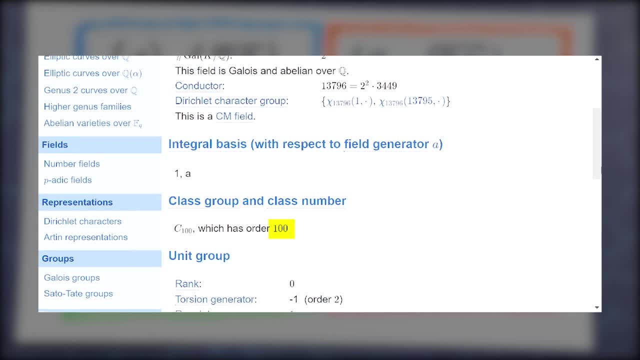 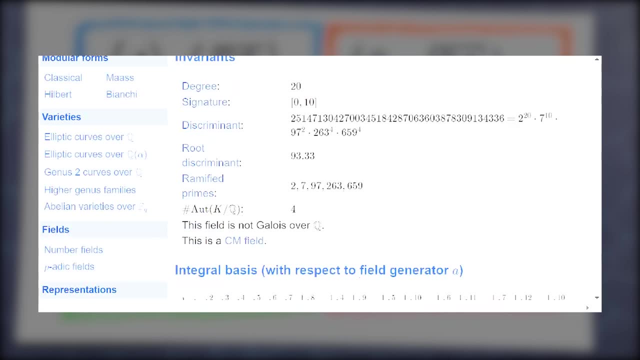 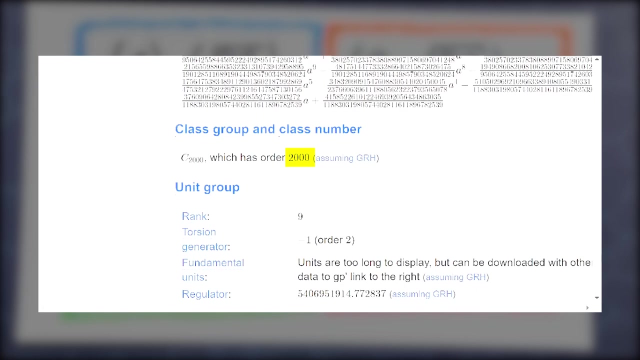 It's very, very complicated. As another example, if you look at the number ring defined by this rather more complicated polynomial, the class number is 2000.. There are 2000 different kinds of ideals in this number system, But by far the most intricate number rings of all are these: z adjoin zeta n. 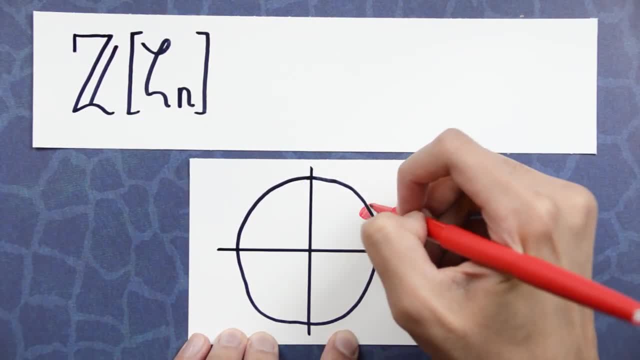 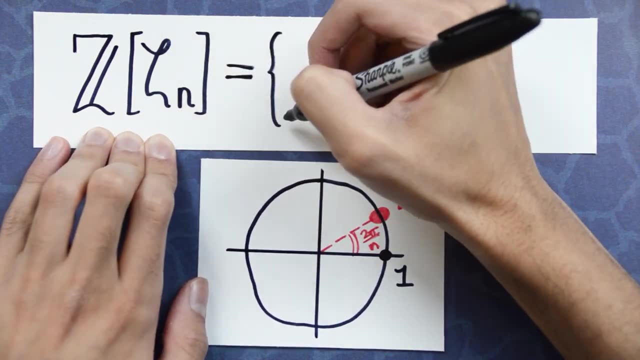 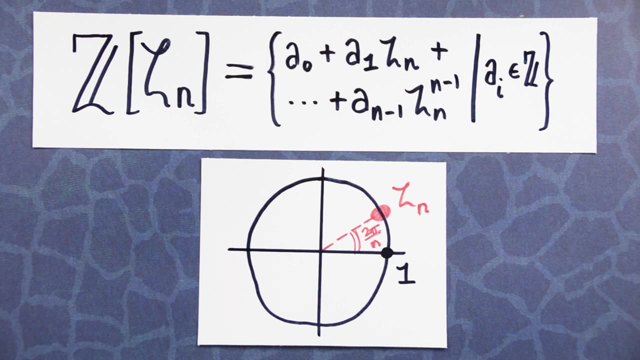 Where zeta n is an nth root of unity, the complex number sitting one nth of the way around the unit circle in the complex plane. This is the set of all complex numbers of the following form. They are a rich testing ground for understanding class numbers. 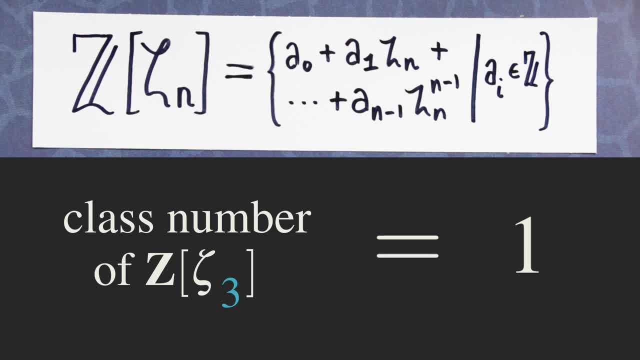 To get a sense of how complicated these can get, here are some examples. For n equals three, the class number is one. For the next few values of n, it's still one. Now let's see how it changes when n grows. 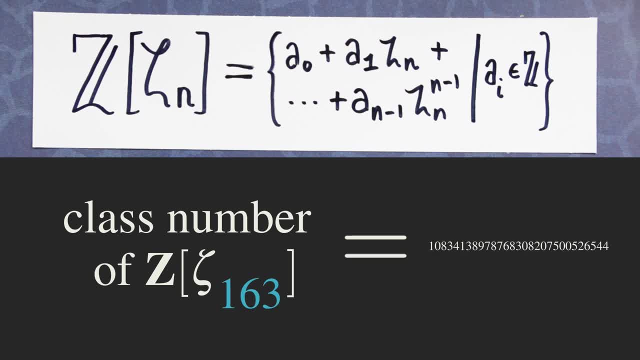 As you can see, it explodes, And I want to emphasize this is not for shock value. These numbers mean something very specific. As an example, in z, adjoin the 23rd root of unity, the class number is three. That means that this ring has three kinds of ideals. 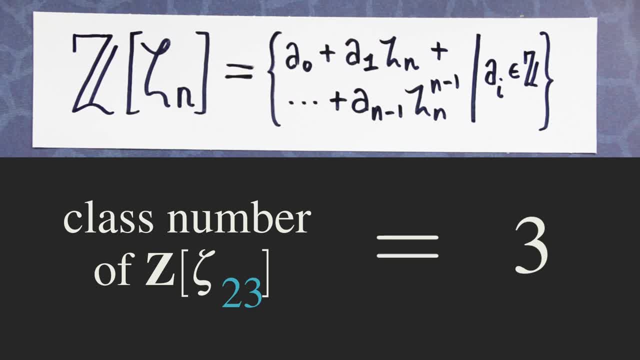 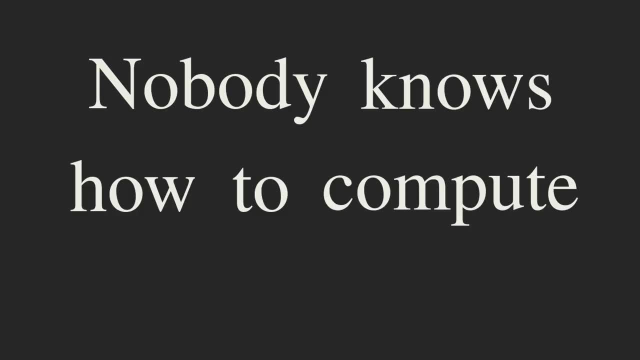 There are three different bandaids you need to apply in order to restore unique factorization in this ring. If there's one thing I want to emphasize here, it's this: Nobody knows how to compute class numbers. They are very, very hard to calculate, even in specific examples. 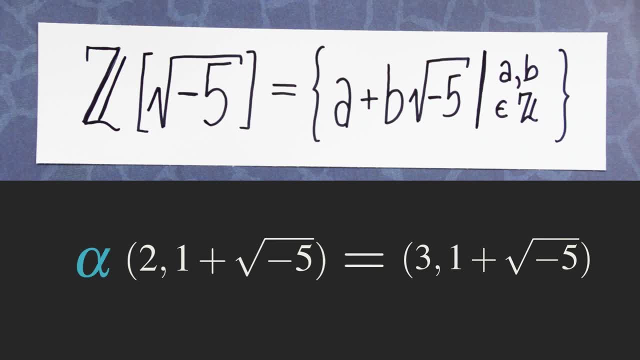 Because to calculate them you essentially have to understand all the ideals in your number ring, Which ideals are multiples of others and which ones aren't. It's a very complicated business. To underscore this, you might have noticed that in the previous example there is a number in the first and last order of the number, that's one, two and three. 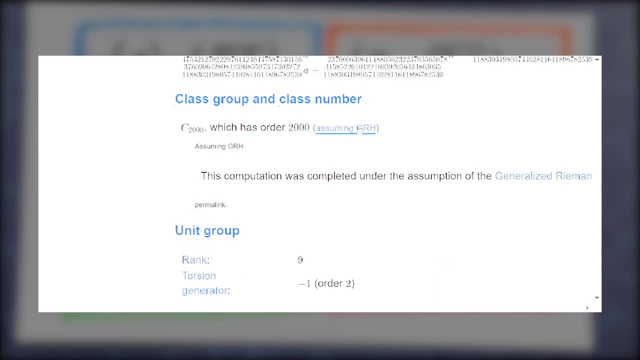 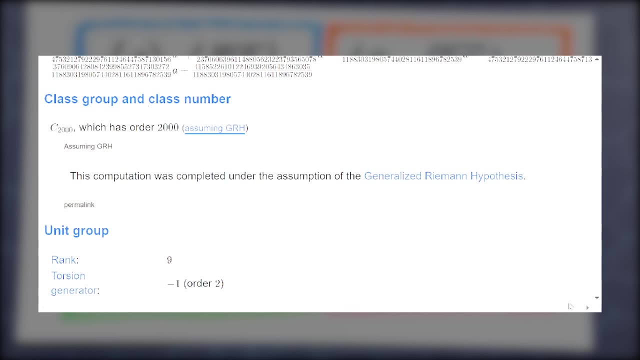 of a class number. it said GRH beside it. This means that this class number was calculated under the assumption of the generalized Riemann hypothesis, which is a very famous unsolved problem. In fact, even for the numbers that I showed here, most of these numbers are also. 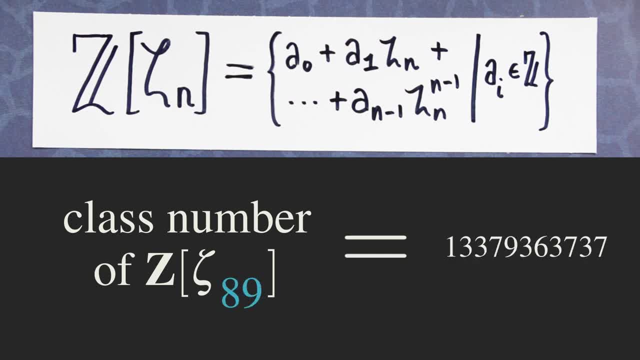 conditional on the generalized Riemann hypothesis being true, The point here is that class numbers are very, very mysterious and nobody knows how to compute them. That all changed in the 1950s, when Kenkichi Iwasawa entered the scene. Instead of calculating the class number of just one number, 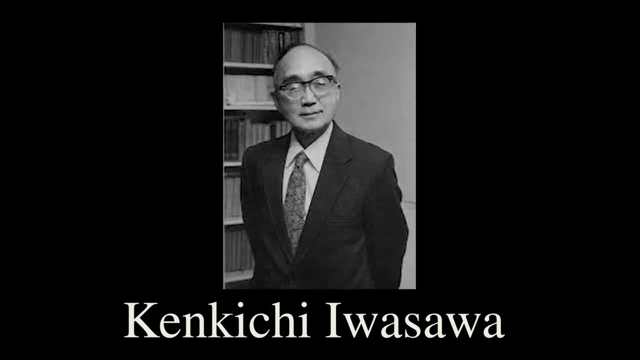 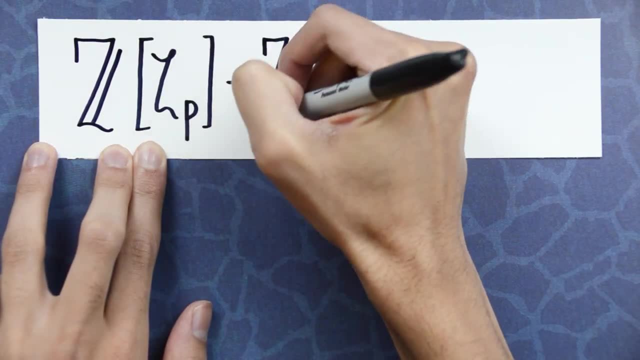 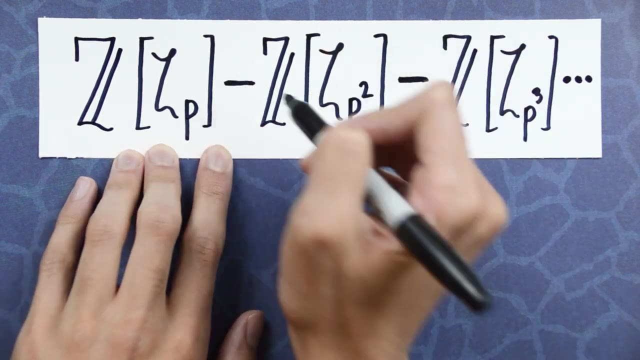 ring. he actually looked at an infinite tower of number rings and calculated all of their class numbers in one shot. Specifically, he considered the following tower: z adjoined zeta p, z adjoined zeta p squared, z adjoined zeta p cubed, and so on for infinitely many layers. He noticed that if 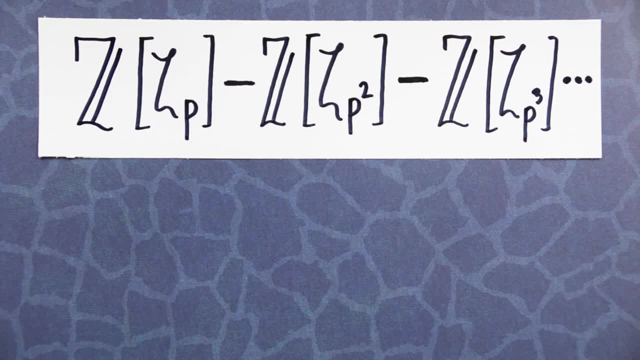 you looked at the class numbers in this tower, a pattern emerged. Take the case: p equals three. this is z adjoined zeta 37, z adjoined zeta 37, squared 37. cubed on and on, forever Finding. 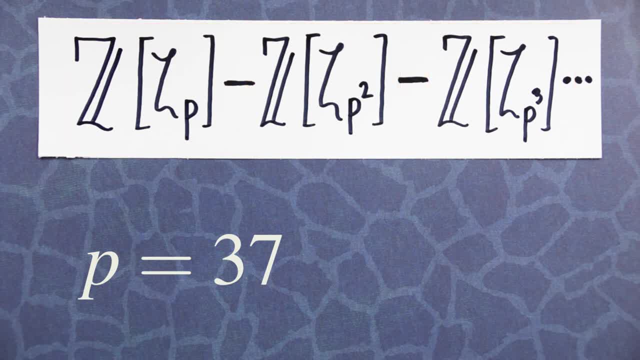 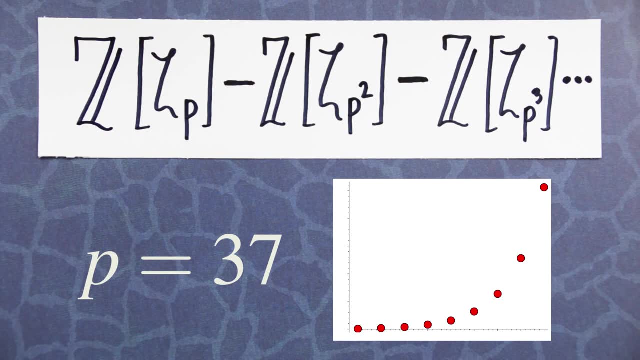 the class numbers of these rings is very hard. but if you just look at the power of 37 appearing in the class number, you see an exponential curve. That is, the power of 37 appearing in the class number increases exponentially fast as you climb the layers of this tower. Take another prime. 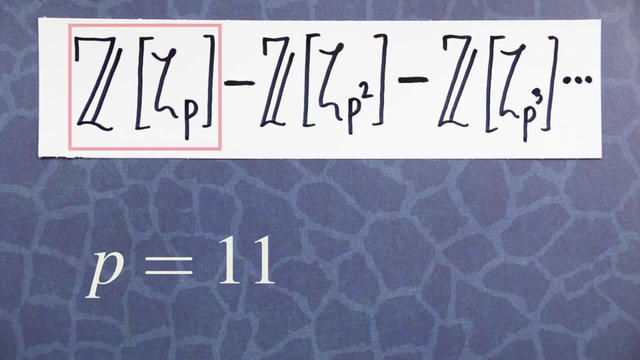 say p equals 11.. So the tower now is z adjoined zeta 11, z adjoined zeta 11, squared zeta 11 cubed on and on forever. Let's look at the power of 11 appearing in the class number. 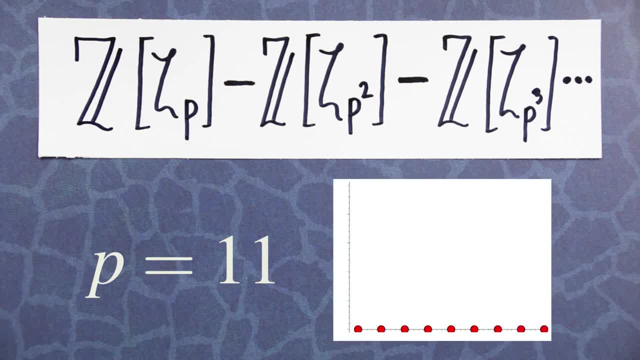 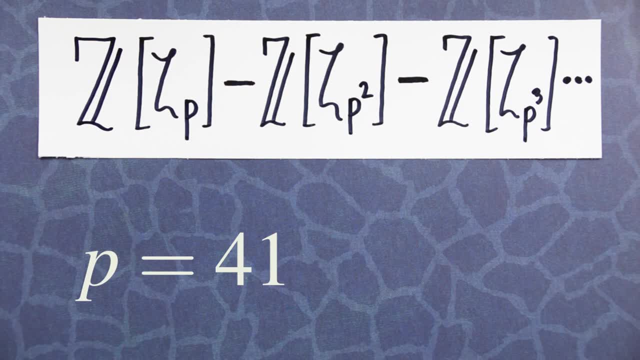 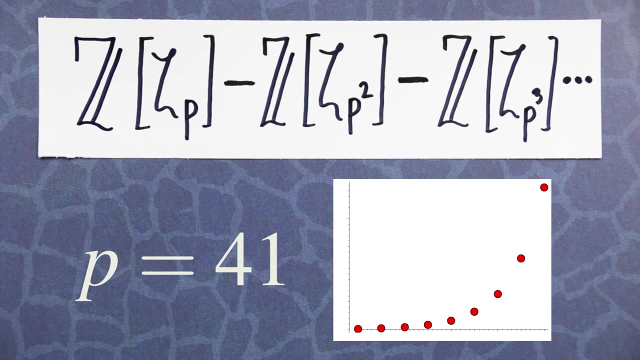 Here it's different. It's actually identically zero. ie 11 never divides the class number of any number. ring in this tower This kind of trend continues. So for some primes like p equals 41, we see an exponential curve. The power of 41 dividing the class number increases. 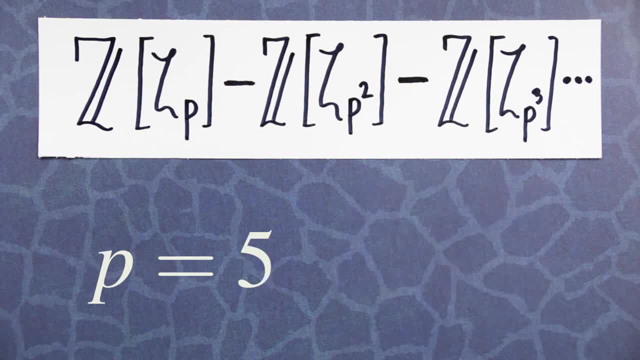 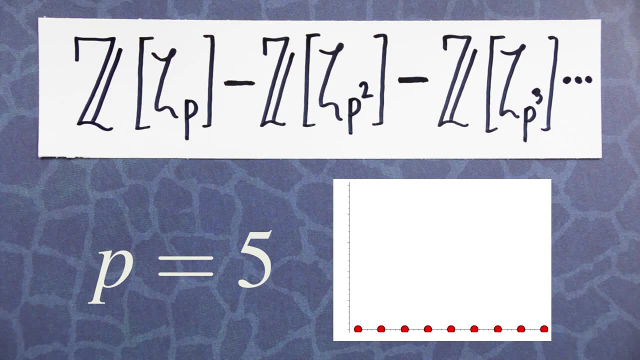 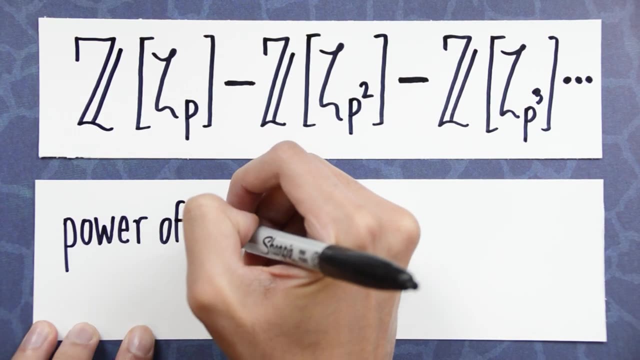 actually. But for other primes like p equals 5, it's a flat line. p never divides the class number of any layer in the tower. This is what Iwasawa was able to prove happens in general. His theorem was the following: The power of p dividing the class number of 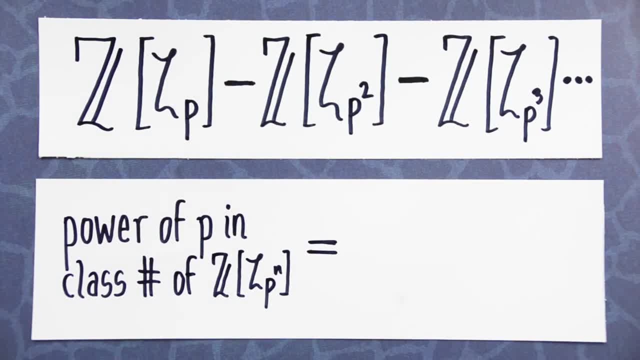 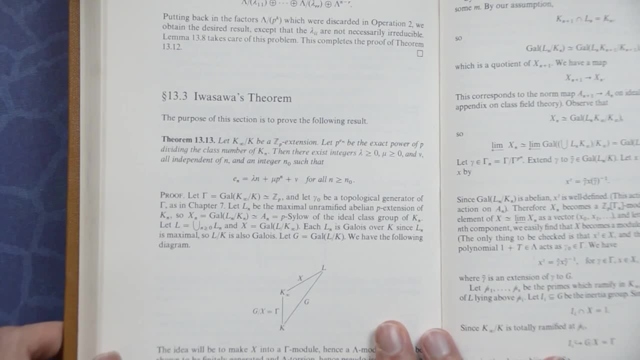 z adjoined zeta p to the n equals p to the lambda n plus nu. for some integers lambda and nu, And this formula is true for every single value of n. The proof of this result is incredibly deep and difficult. It uses some very sophisticated 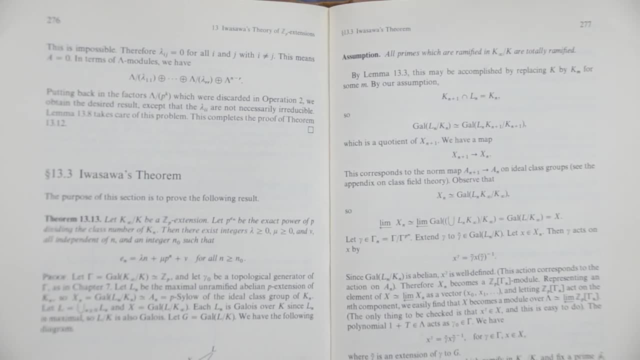 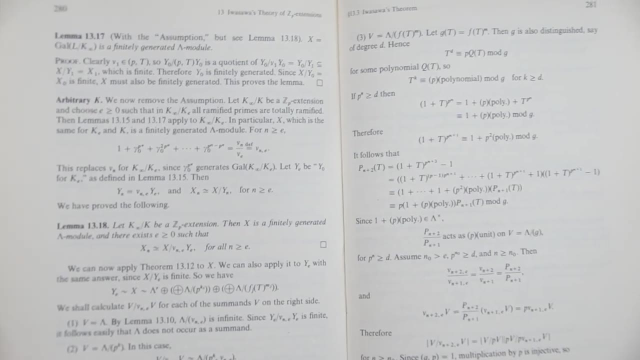 tools: Group theory, representation theory, class field theory and much more. The basic idea is that if you arrange these rings in an infinite tower, you can look at all of their ideals at once, And this object has many more algebraic symmetries than the ideals. 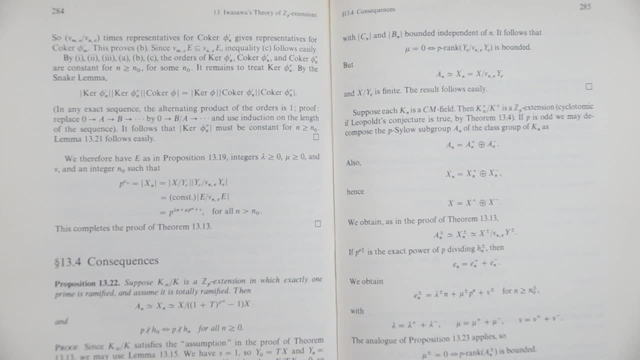 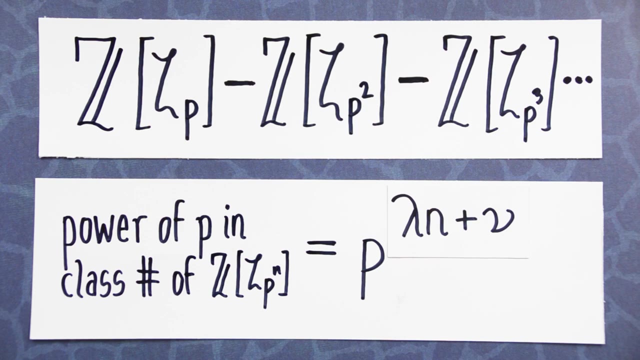 at any finite layer. The strategy was totally groundbreaking and nobody had seen anything like it before. Unfortunately, the theorem as I've stated it, however, isn't quite correct. His result actually had an extra term mu p to the n for some integer mu And unfortunately this error term was 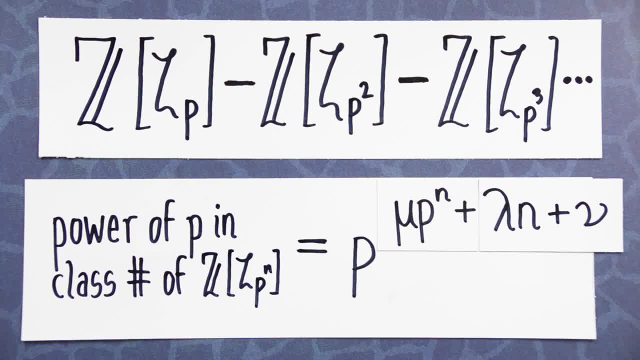 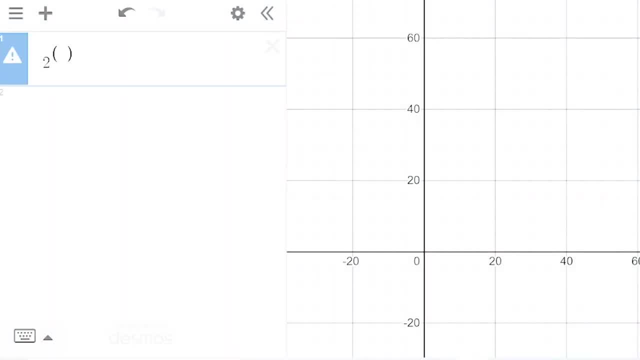 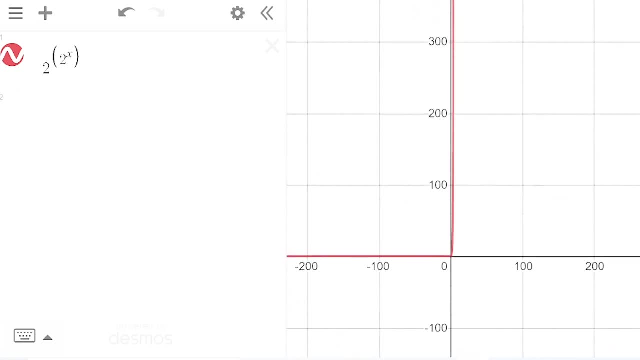 absolutely gigantic. It was an exponential of an exponential And it completely overshadowed the main term. To get a sense of scale, if you graph 2 to the 2 to the x, you'll notice that the x-axis explodes very fast. It almost looks like a completely vertical line. 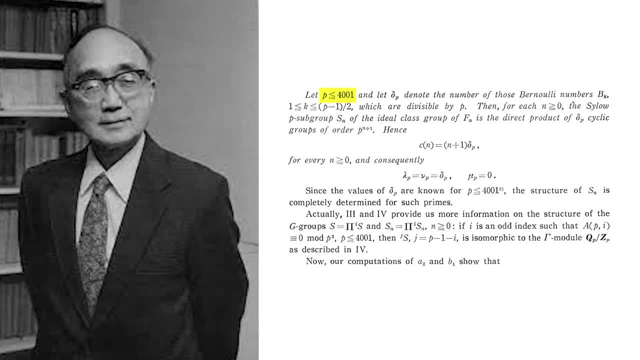 In numerical computations of these class numbers, Iwasawa noticed that for all primes less than 4009, mu was always equal to 0. That is, this term wasn't actually there, But it turned out to be very difficult to prove this for all primes p, And it took almost thirty years. 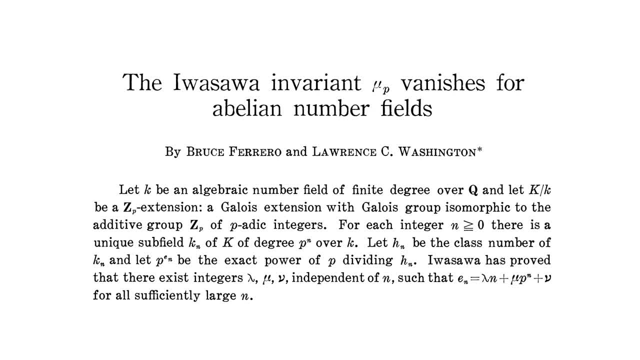 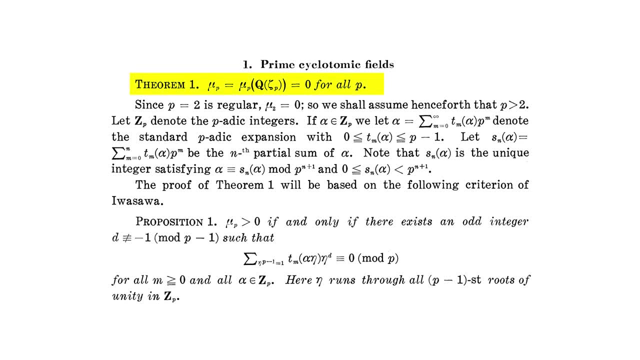 And this was finally proved in 1979 by Ferrero and Weiss. They proved that for all primes p the mu-invariant of the p-th cyclotomic field was zero. But with this theorem in place, we could then remove this extra term and get the thing. 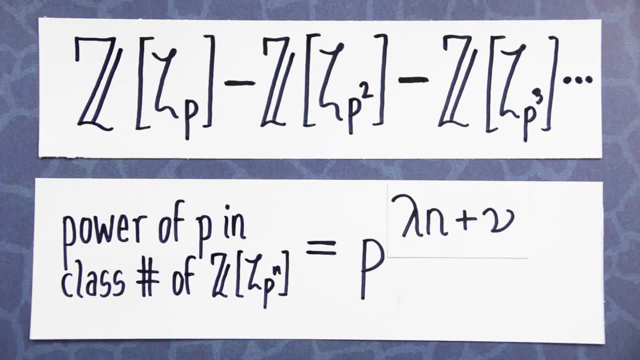 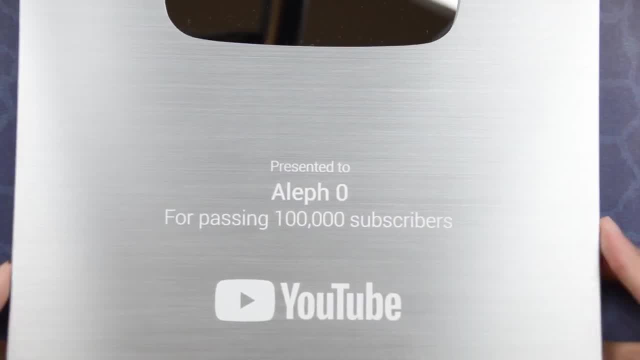 that we observed in all the data. That officially ends the math part of this video. I wanted to finish with a thank you. This channel recently hit 100k subscribers and I wanted to thank you, dear viewer, for choosing to spend your time learning math with me. Thank you so much for watching and. 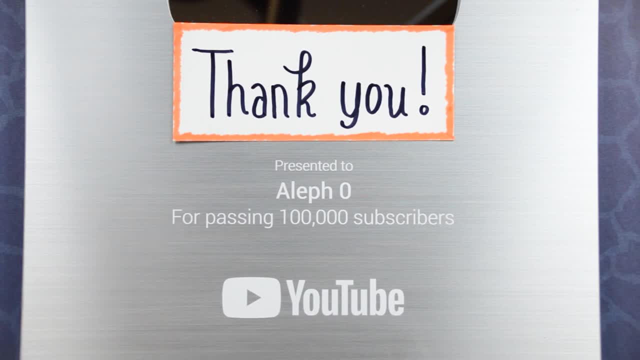 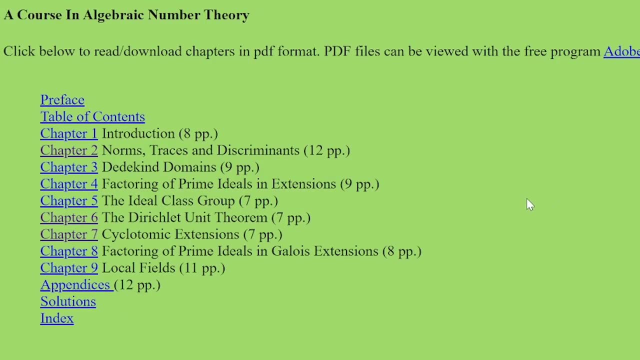 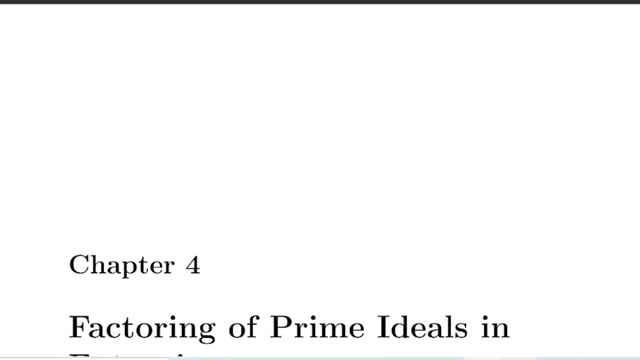 I'll see you in the next video. In conclusion, I'd like to list some resources to learn about this stuff rigorously. For algebraic number theory, there are tons of online notes from which to learn the subject. My personal favorite are these notes by Professor Ash from the University of Illinois. Personally, 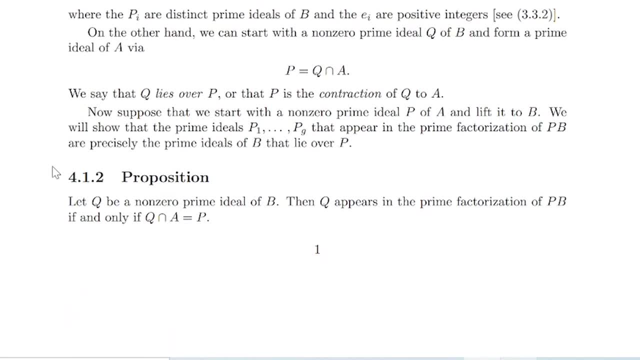 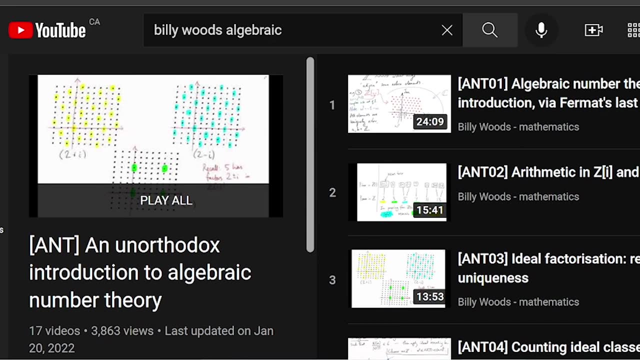 I tend to like notes that have lots of numerical examples because they really make you feel like you're seeing the real phenomenon, So these notes were good to absorb the main contents. If you're more of a videos person, there's a nice video playlist that you can download. 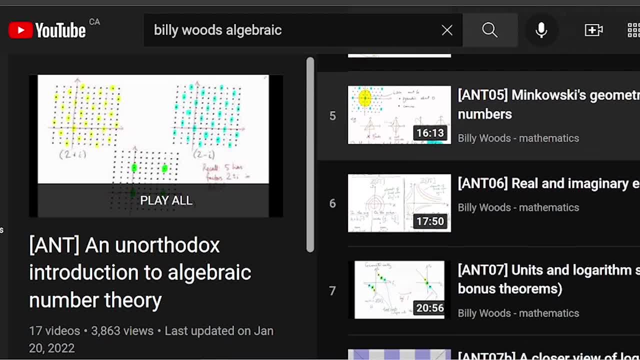 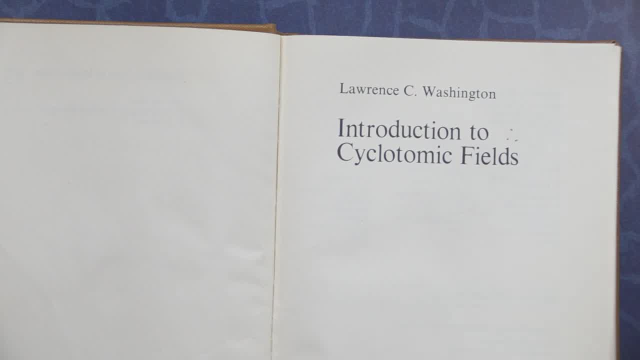 It's by Billy Woods which covers all the main topics. The link is in the description For Iwasawa theory, the bible for learning. this is by far The Introduction to Cyclotomic Fields by Lawrence Washington. And yes, this is the same Washington who proved mu equals. 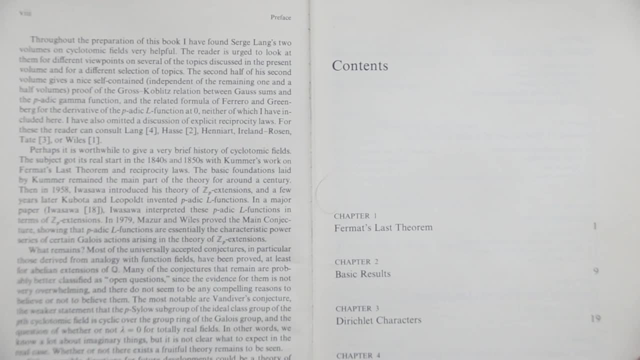 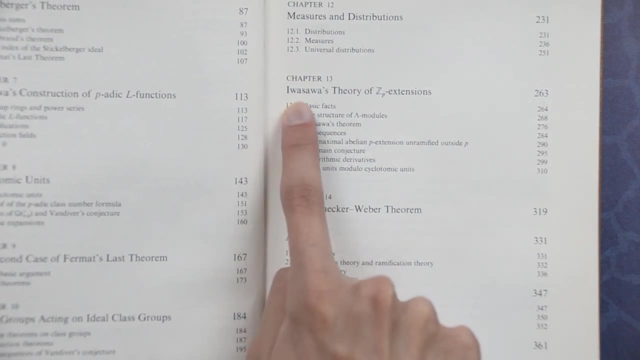 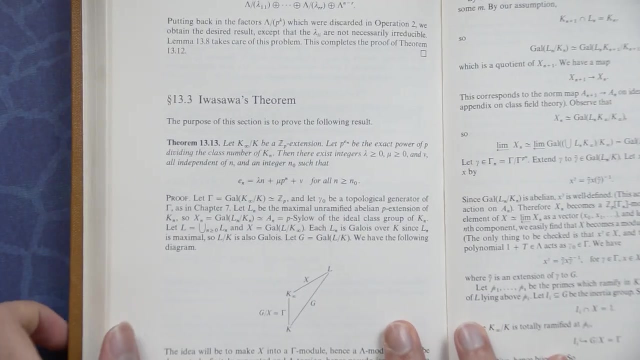 zero. This book is a graduate textbook so it is terse and it requires a solid grounding in algebraic number theory. The theorem that we saw was from Chapter 13, Iwasawa's Theory of Zp-Extensions. This book contains a full proof of this miraculous theorem. It's complicated but undeniably beautiful. 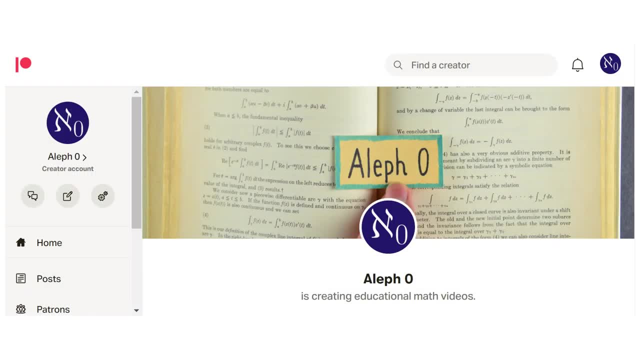 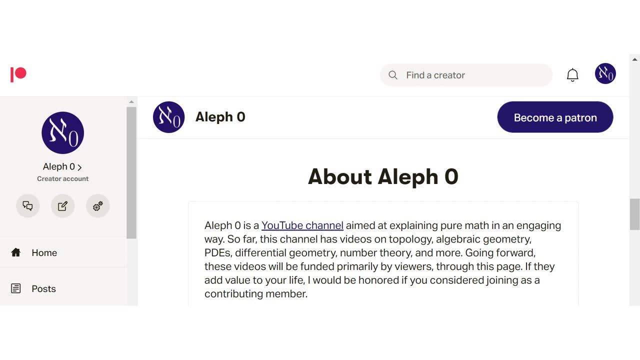 An announcement for the channel. Aleph Zero now has a Patreon page, So if you enjoy watching these videos and they add value to your life, I'd be eternally thankful if you'd like to support the channel on Patreon. All the links are in the description. 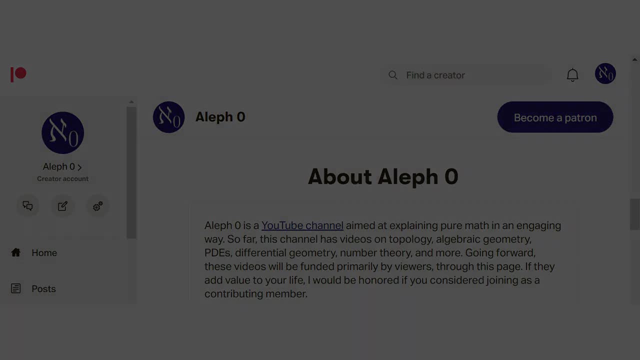 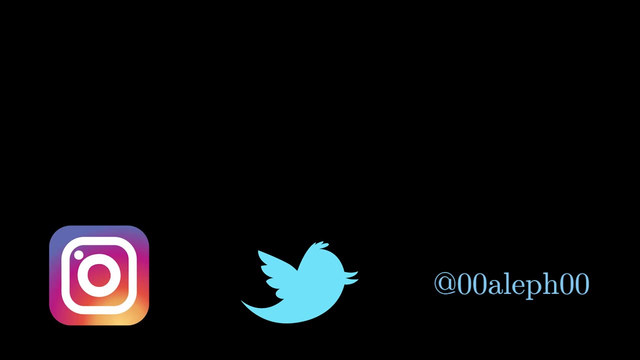 That's all for now. Thanks for watching and I'll see you next video. Bye, Bye.